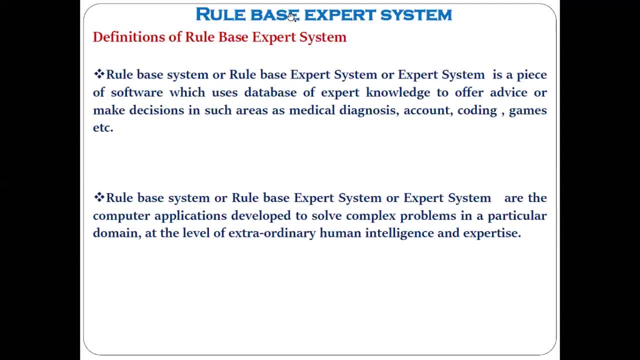 kind of symptoms that you are having. but the doctor perform the checking And if you have the symptoms like the fever, headache, vomiting, body ache, sweating, okay, So these are the symptoms of the disease malaria, Okay, Okay, Then the doctors tell you that we have the disease malaria and you need to take some. 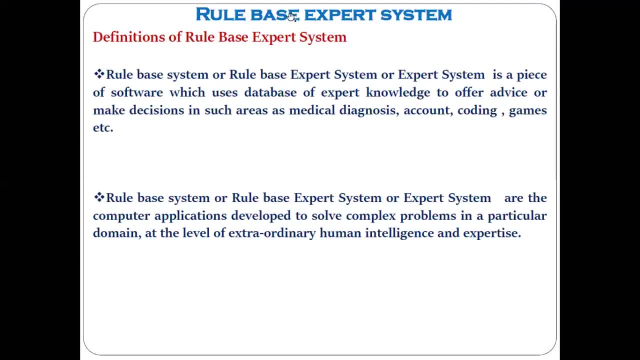 precaution and the treatment. Another case suppose: if you are the, if you see the current situation and if you have the symptoms like the, for example, high fever, sore throat, sore throat, sore throat. okay, Gasa Corda. 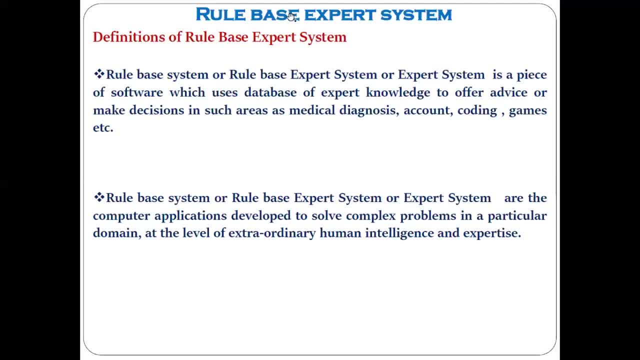 You have the breathing problem and you are feeling the tiredness, Then these are the symptoms of the disease Corona, So that to tell you, you have the Corona. Okay, Now how does the doctor know all these things? And how does the doctor making such kind of decision and telling you? 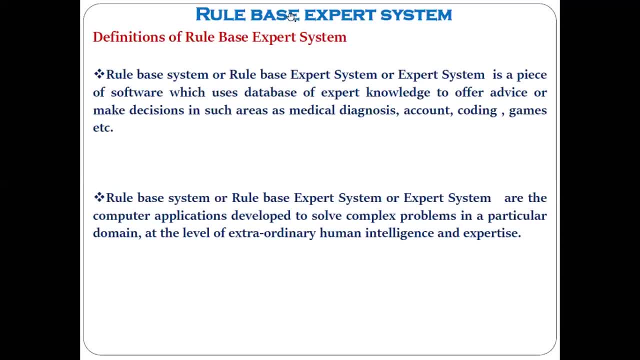 That is my question to you. Yes, All of you understood the question. Okay, Yes, Yes, How does the doctor know all these kind of things Really? Yes, Okay, From the period we all started the lecture, I don't heard your voice clearly. 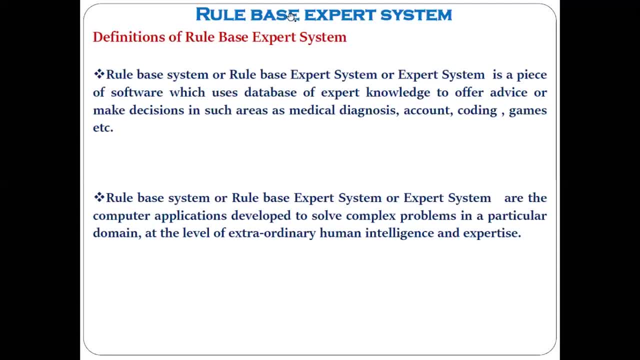 Try to be in the okay Good range area. Hi, How does it is possible for the doctor- Okay, Yes, Yes, Yes, Yes, He knows about the all the symptoms of Corona. All right, That is I'm asking. 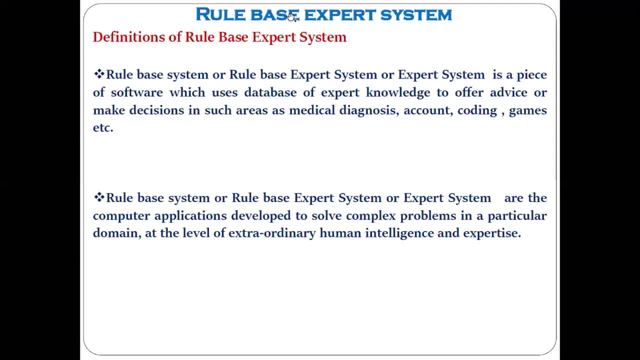 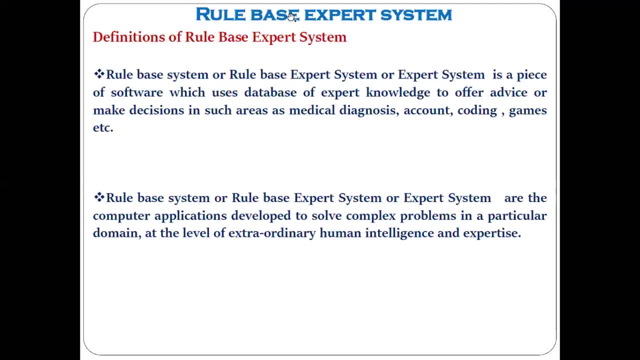 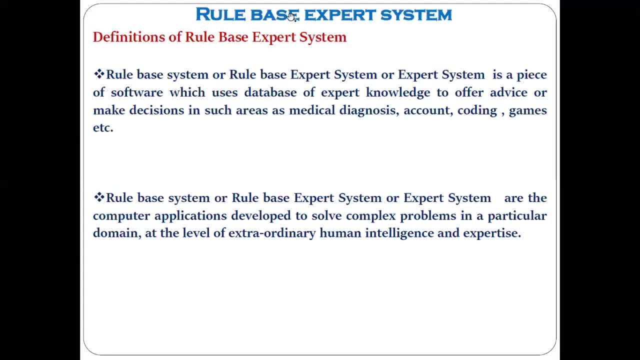 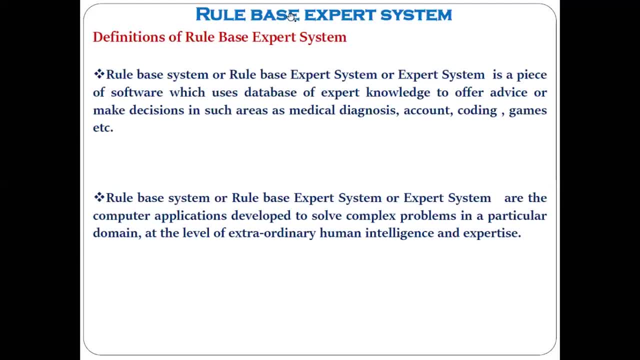 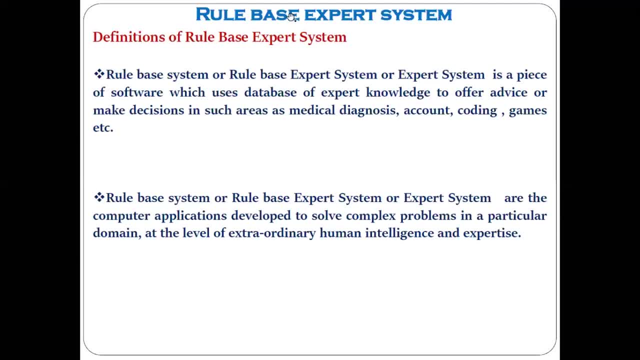 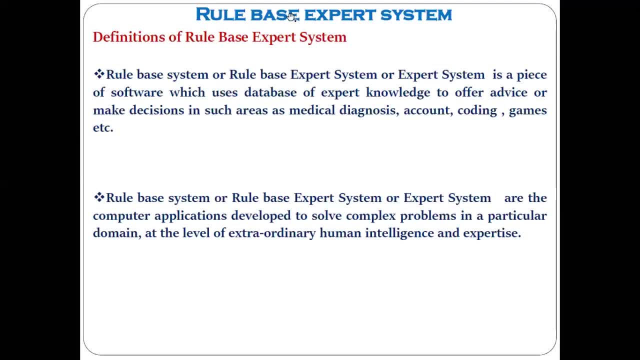 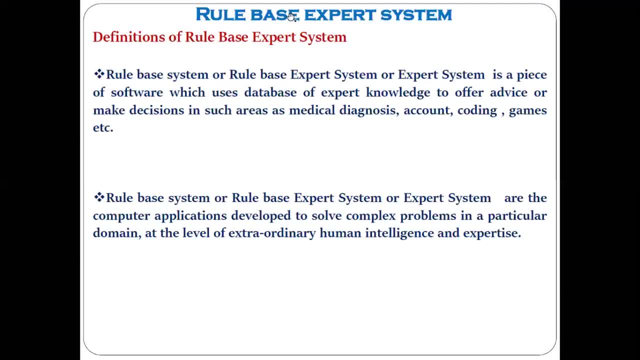 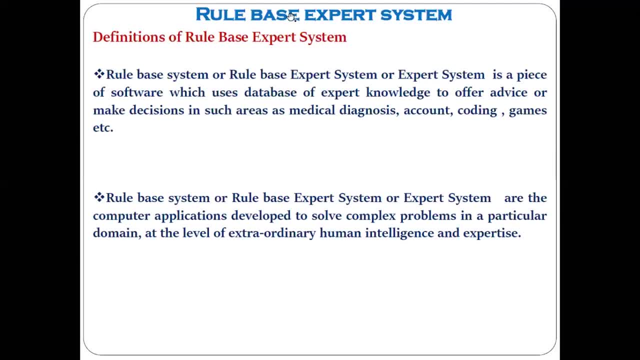 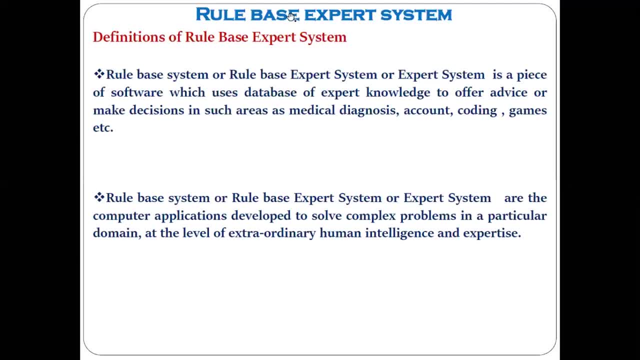 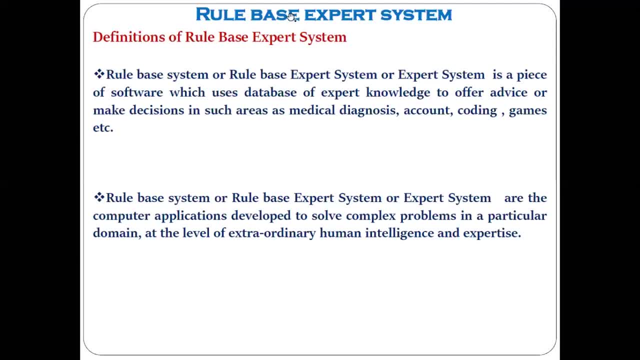 doctor as a physically doctor, natural doctor as a- we are calling him as a rule based expert system. that much is understood. what I am asking now: we want to develop a non-natural system which will behave like the doctor. Now, in order to do that, what has to be done? 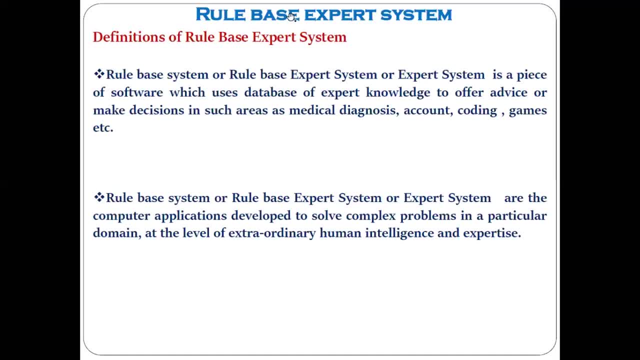 Non-natural doctor which will be like the natural doctor, which will can take the decision, like the natural doctor, which can give you the, which can apply the rules, like that kind of things, and can give you the some kind of output. Okay, Then, what has to be done? 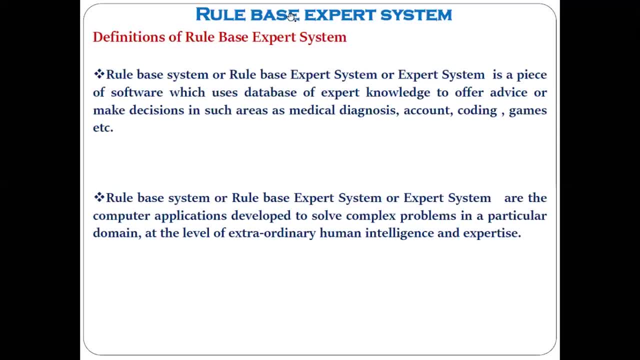 Non-natural system where to develop, Then how it can be developed. I think we have to install different probabilities in it, that if the patient has normal cold cough, then what medicine should he take? If you want to make something non-natural, then the simple thing is nothing, but you can. 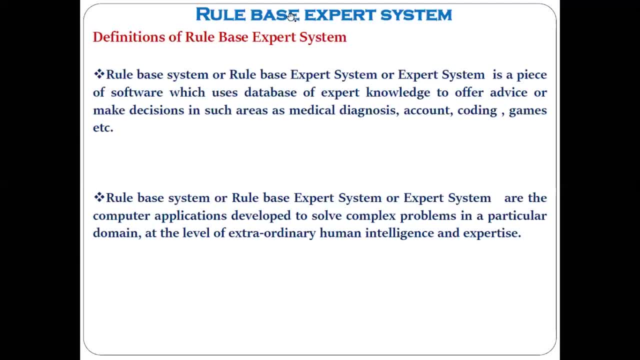 do it only through the intervention, Integration of hardware and software, etc. correct or no? Yes, different installations will have to be done in it. He has total knowledge about this. Yes, yes. so what we have to develop if you want to develop the non-natural doctor which 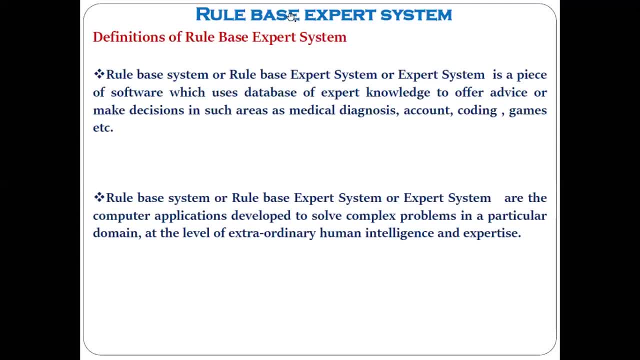 can behave like the same natural doctor, you have to develop one software system with the integration of some hardwares, yes or no? Yes, sir, And that is nothing but called as a. Now, If you want that non-natural system should behave like the doctor, you have to put some. 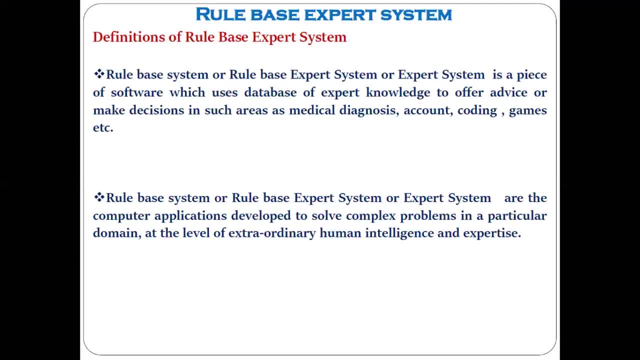 knowledge within that? correct, Because natural doctor already has taken the degree. that's why he has got the experience, etc. etc. But if you are trying to develop the non-natural system through the programming, we need to put the knowledge within that system, correct. 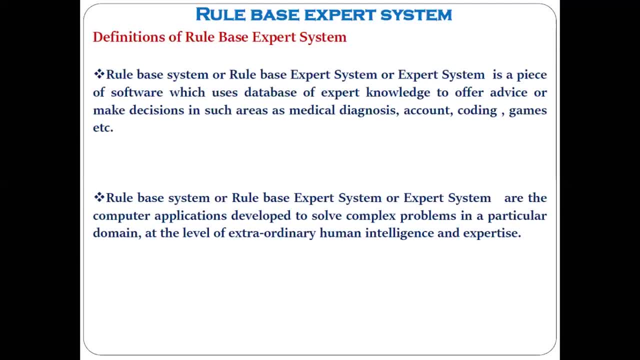 Yes, You need to also write the program so that that system can apply the rules. that system can perform the comparison and give some result. correct, Yes, sir, You need to write some programming code there so that that system can understand when some 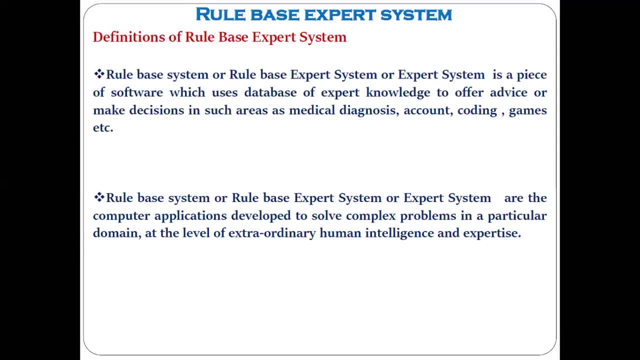 person ask question to that system, correct? Just like you are asking question to our physical doctor, correct? Yes, sir. So these all things has to be developed, Yes, sir. And then we can have the non-natural doctor, which can behave like the natural doctor. 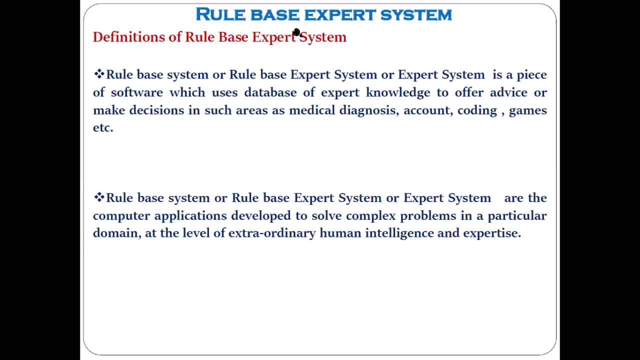 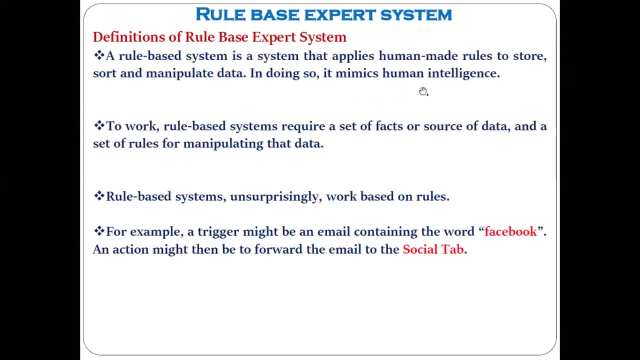 And that is nothing but the called as what. that is nothing but. our today's point of discussion is what? Rule-based system, or rule-based expert system, or the expert system, It is what. It is simply the what is what it is. it is simply what. 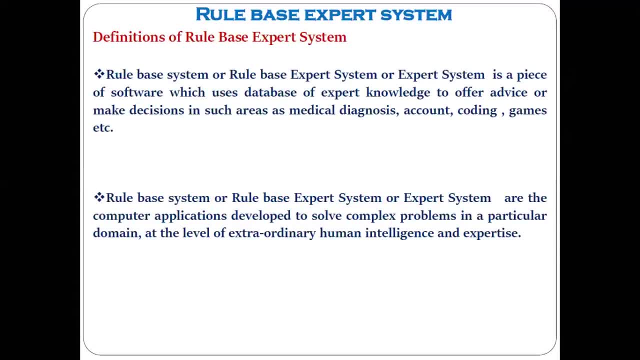 Human intelligence. It is simply nothing but putting the human intelligence in some particular system. understood So that rule-based system or the rule-based expert system is nothing but what It is: a kind of software which uses what. It uses some database of expert knowledge to offer the advice or to make the decision. 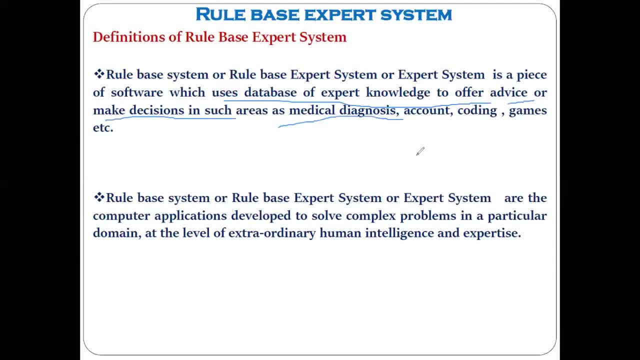 in various areas Here. I have just mentioned some areas like the medical diagnosis, accountability. Yes sir, Yes sir, And that is nothing but the code. as what? the rule-based system or the rule-based expert system? Do you understand? what does it mean by the rule-based expert system? 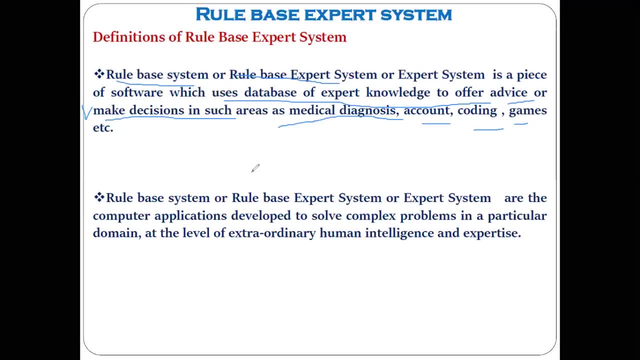 Yes sir, Yes sir. So that's why I have taken first the natural rule-based expert system example and the same example we have applied to the non-natural Understood. Yes, sir, So that's another way which you can describe the rule-based expert system, like rule-based. 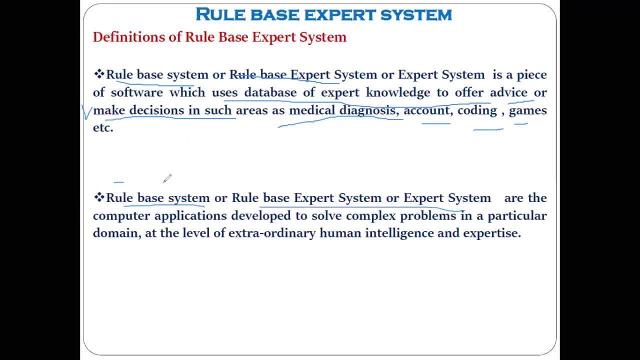 system, or the rule-based expert system or expert system. I have used these three terms because in the exam the terms can be different. Okay, So that you don't get confused. This rule-based system are nothing but the kind of different computer application developed. 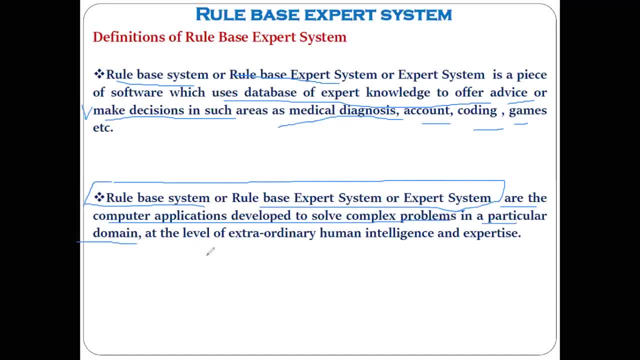 to solve the complex problem in particular domain, at the level of extraordinary human intelligence and the expert pile. Yes, sir, So you can call the any computer application which is solving some complex, complex problem and while solving the complex problem, that computer application applying the same intelligence that human apply in the real life understood. 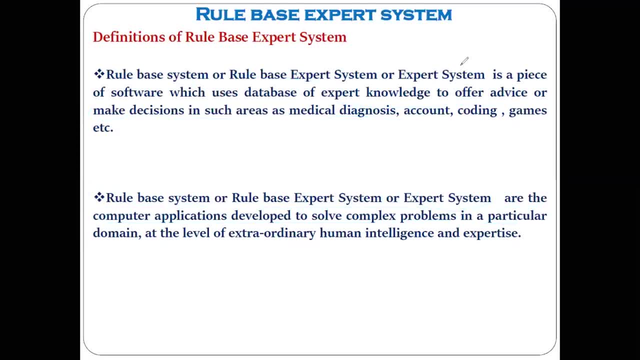 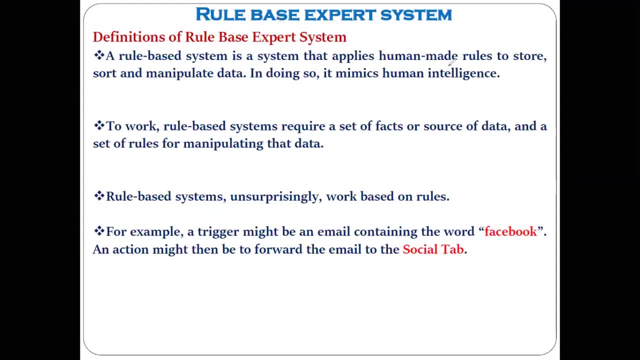 So this is also the another way to describe what is mean by the rule based expert system. Here also I have written in the another words. like you can see here, the rule based system of the rule based expert system is nothing but apply the human made rules to storing the knowledge, sorting out the knowledge or comparing the knowledge and manipulating the data, in the sense processing the data so that he can copy the same human intelligence. 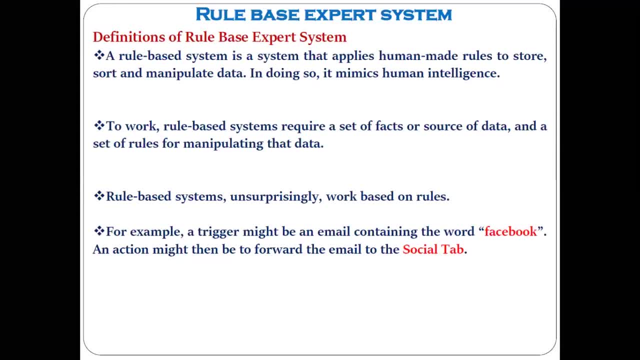 Understood when you are trying to, when you are developing the non natural rule based system There is, There you have to store some, as I said, you, with the help of some programming language, there you have to store some rules understood, there you have to store some knowledge. there you have to, there you have to write the some programming code so that with the help of that programming code, that data or knowledge which is being stored there in the, that database, that get compare and we can get the result, just like the doctor is giving, the result related with the after checking various kind of 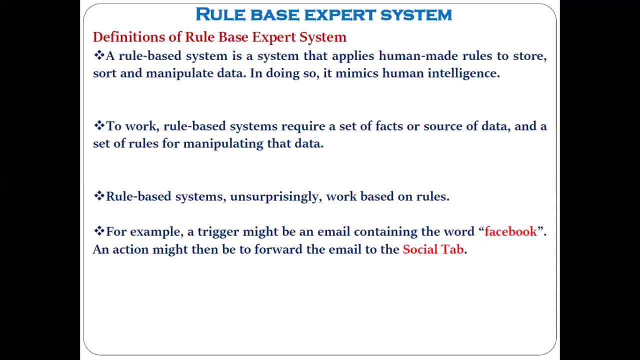 After checking the Different kind of symptoms, sense and giving the output that what kind of this is you have understood? So now, just like the human being, as a doctor, it requires the some kind of knowledge of some fact or the sources of data, and then he applies some rules on that sources of data and give the result. in the similar way, in the non natural rule based expert system, which is nothing but the application of the artificial intelligence. there also need of this. 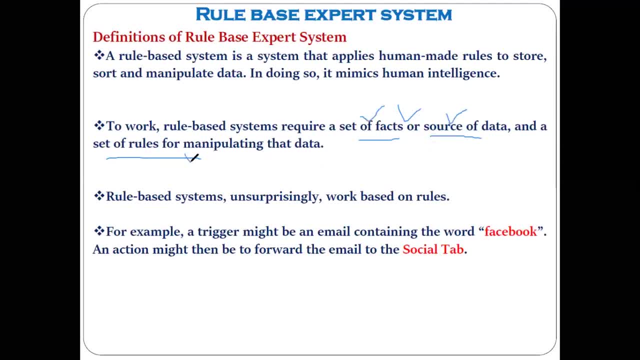 So with these things, fact, source of data, set of rules, etc. It's it now how we are making all this thing possible in the non natural rule based expert system: by by, by developing some soft, by integration of some software and hardware, by utilizing some programming language, etc. etc. understood. so, in short, can I say: the rule based system work based on the rules. 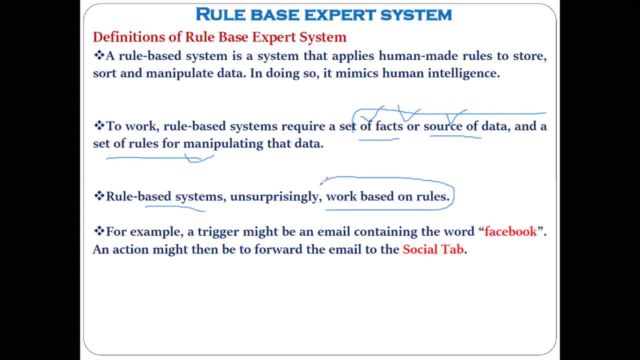 So, in short, can I say the rule based system work based on the rules, correct? that is the reason it is be referred as a rule based system. the way you write the rule in that system. accordingly, that that system will work yes or no, correct? yes, sir, yes, so that is the. it is working on the basis of the rules. that is the reason it is being 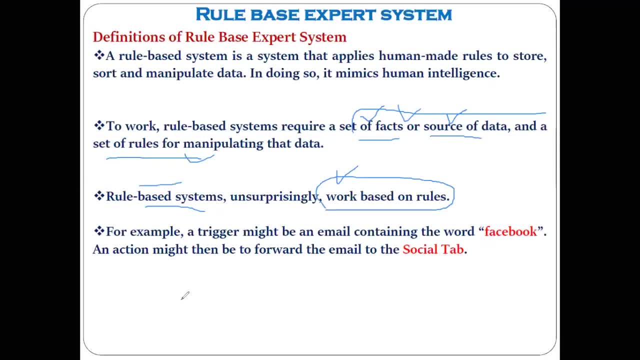 referred as the rule based system. now, in the general life also, we can take the example of some rule based experts. rule based system. like you can say, your gmail can be also called as a rule based system, yes or no? how can anybody tell me? gmail can also be called as a rule based system. 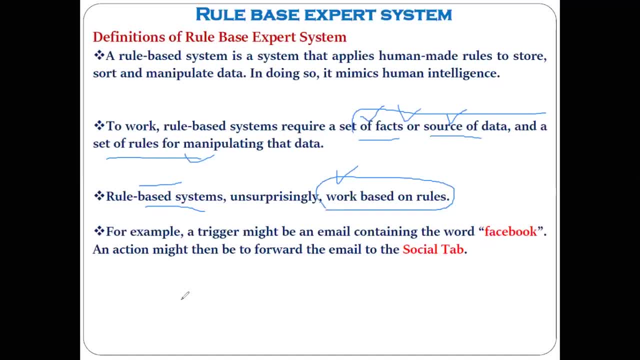 how- yes, to understand the question, how we can call the gmail as also rule-based system and it also tells us that you got the mail. now, that is not the example. i'm calling the gmail as a rule-based system and i'm asking how we can call like this to the gmail. 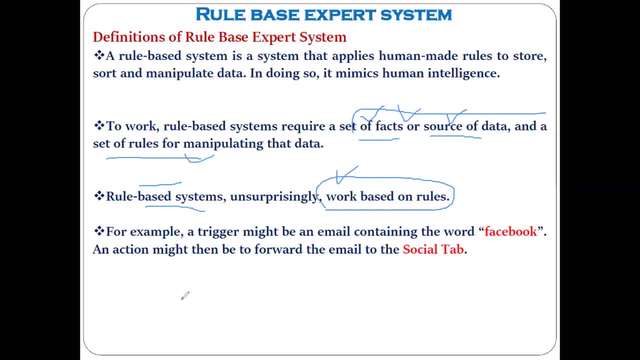 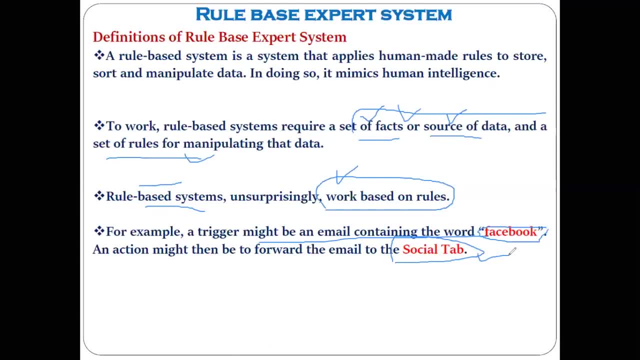 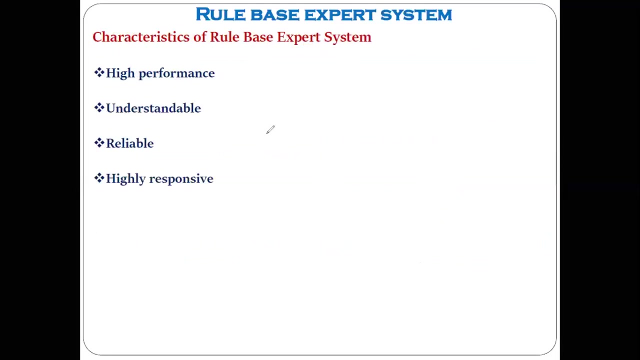 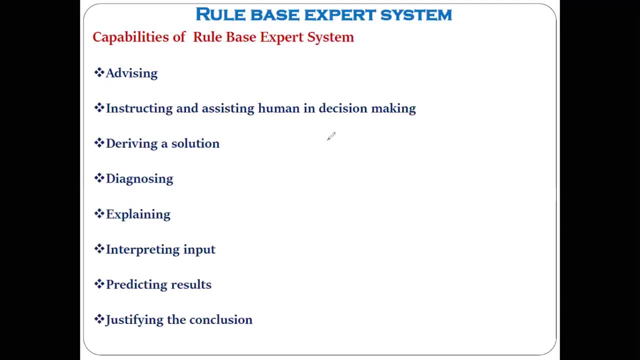 carrying the example of physical doctor as a rule-based system and the non-natural rule-based system. yes, so in the, if you take the example of physical doctor, also natural doctor, he can give you the advice. same way the non-natural rule-based expert system also can give the advice. it can. 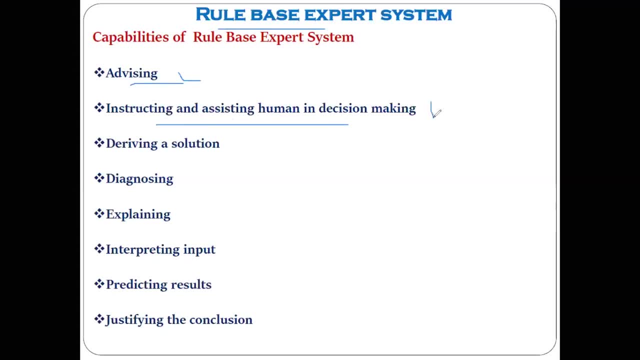 help to make the various kind of decision. okay, it can help you to get the solution. it can help you to for the diagnosis purpose. it can help you to explain the reason behind certain kind of advice. now, if you want certain output from the expert system, first thing is what you need to give some. 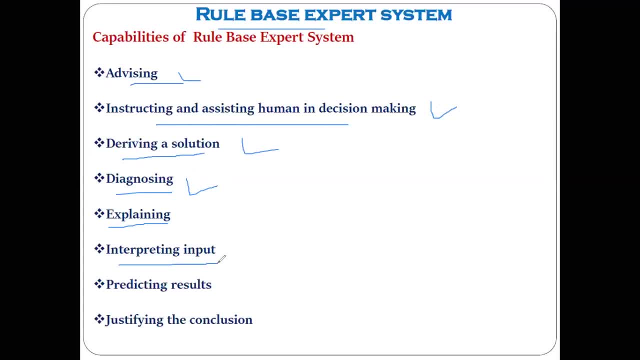 input correct. just like in the natural doctor thing, you, until you not tell your doctor that doctor I have, I am feeling these kind of things, etc. etc. that is nothing. but the input till that doctor will not tell you what, what this is you are having, yes or no? yes, 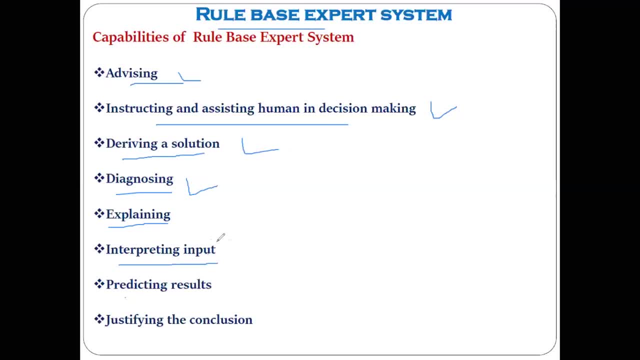 so non-natural rule-based expert system can also interpret the input, it can also predict the result and it can also give you justification for your whatever the output it is giving. so all these capabilities are there in the rule-based expert system. now main point: that is nothing but what. 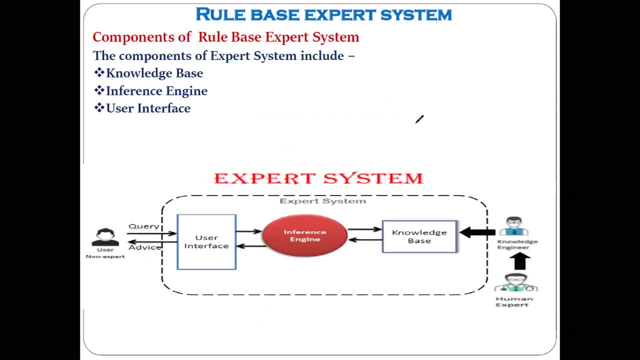 are which are the different components on the basis of which the rule-based expert system works? mainly, there are the three components: the knowledge base, inference engine and the user interface. this is the diagram for this very important okay. this diagram you can see easily. I have shown you here. 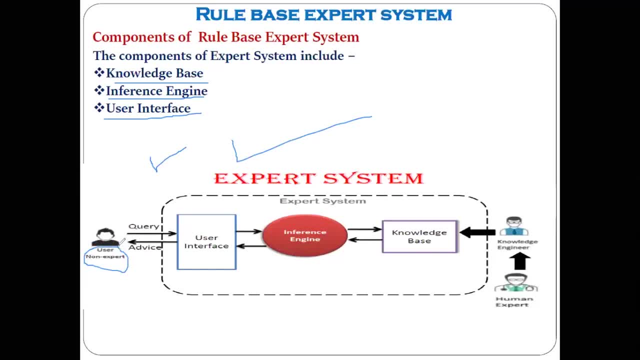 user. I hope all of you can able to see it clearly. yes, sir, here I have shown the user as a non-expert. when you apply circle as a, we can see the patient where you can call it the patient, for example. okay, now we are where we are trying to discuss this expert system as a medical expert system. okay for. 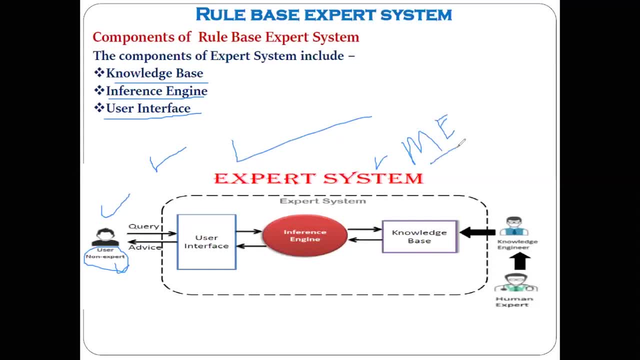 the purpose of understanding, okay, okay, okay. now here, doc user as a non-expert or the patient does some query. yes, it does some query. now, how we can now, when you go to the doctor, how you do input to the doctor, that is my question to you. 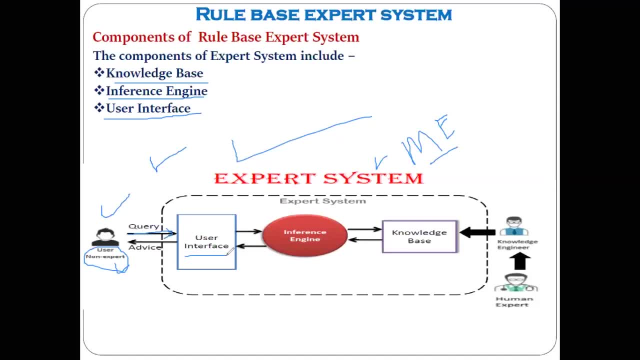 how you give input to the doctor symptoms? are you tell doctor, doctor, I am feeling this kind of things, etc. etc. correct, yes, the user interface, for that is nothing but what. you are using some natural language, correct? yes, sir, that is nothing but your user interface. user interface: nothing but the, the media using which you are. 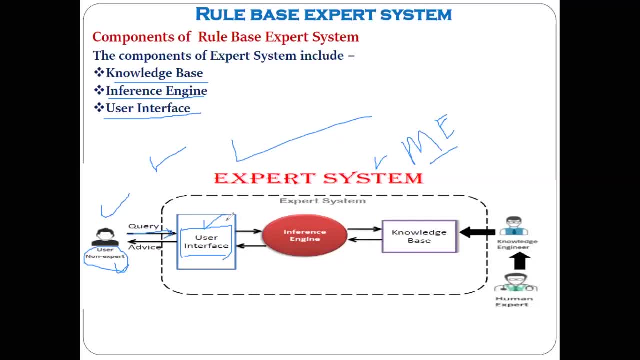 telling something to the system. what the point? yes, sir, great, okay, so before we move ahead, before we move ahead, you do not have to go to the, to the. then, then that you are query, that your query goes to the inference engine- that is the second component understood. then from that inference engine goes to the knowledge base and then again from the knowledge base the reverse journey to the user and the non-expert. understood now, before we, before we discuss about the, 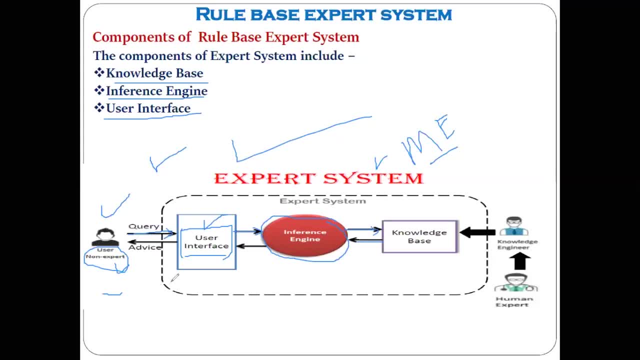 therefore understood. now, before we, before we uh, discuss about the uh, this particular thing, we need to understand what exactly mean by all these components. then we'll discuss the same example. okay, now, what exactly is the knowledge base? now, you- you are now in the final year- you must be having idea about these kind of things, and i'm not, uh, i'm not expecting. 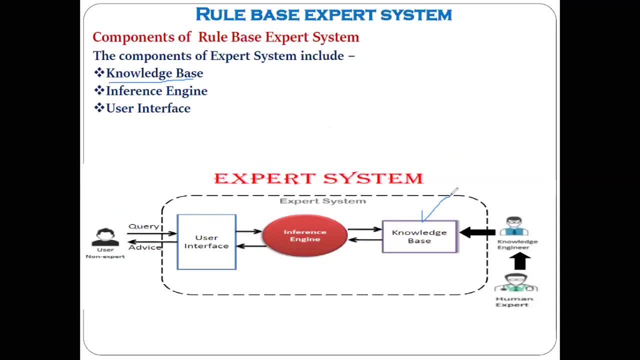 the correct answer from you, but i'm expecting something from you, understood. you should speak up now. you tell me what does it mean by the knowledge base, the first component of the rule based expert system? data collected from previous experience- exactly very good. yeah, just like after taking the degree. also, he need to do the practice. 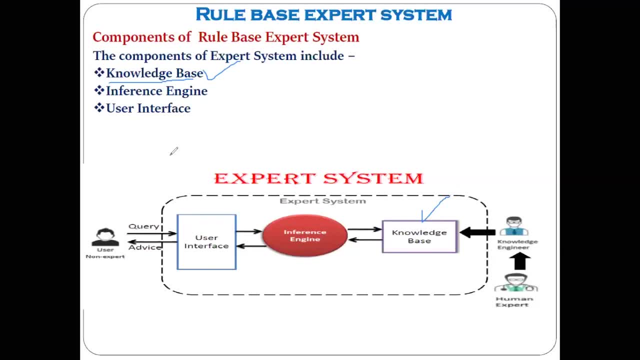 yes, and from that he, he gathered the knowledge and that become his knowledge base. correct, yes, sir. non-natural rule based expert system: correct? yes, now, in that case we have to gather the knowledge from the different sources. expert, correct? non-natural here. we can't teach non-natural from the college. 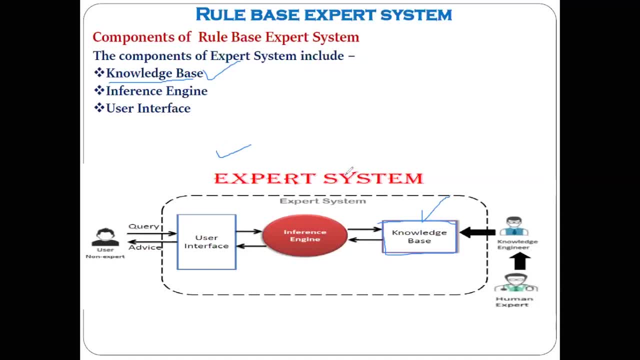 you need to gather the knowledge from the various expert. that various expert can be the human expert, yes or no? yes, sir, understood. now who will gather this knowledge when you are, when you are developing the rule-based system and in specifically non-natural rule-based expert system, who is, who is gathering all this knowledge? there is a knowledge engineer. 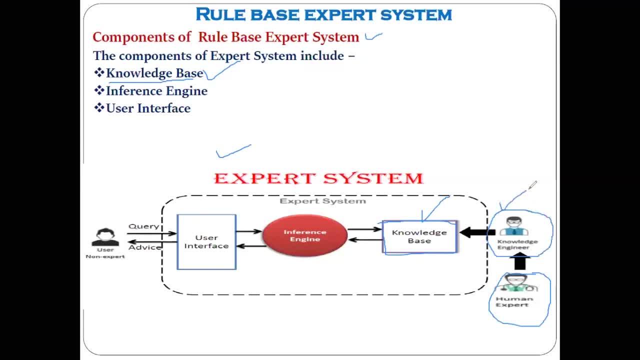 now this knowledge engineer? you can simply call him as a programmer, yes or no? yes, yes, so this knowledge engineer does what: it gather the sources of data it gather. it gather the knowledge from the various human expert, as you are taking the example of medical. it take the advice, it take the help. 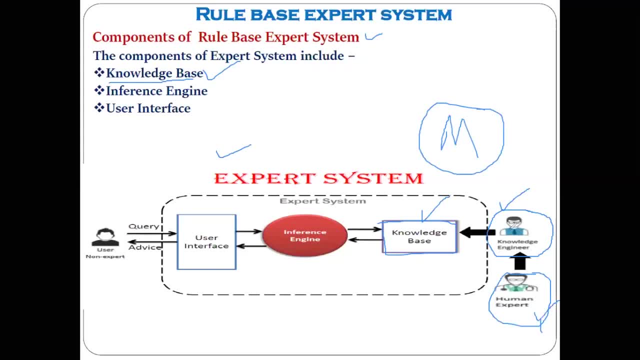 from various human expert doctors and then it gather the knowledge, okay, related to the various kind of disease. understood expert system can be built for the single disease, yes or no, or rule-based expert system can be built for the knowledge multiple disease, all of your agree. so we, we assume here this knowledge engineer: gather the knowledge from various doctors, md mbbs. 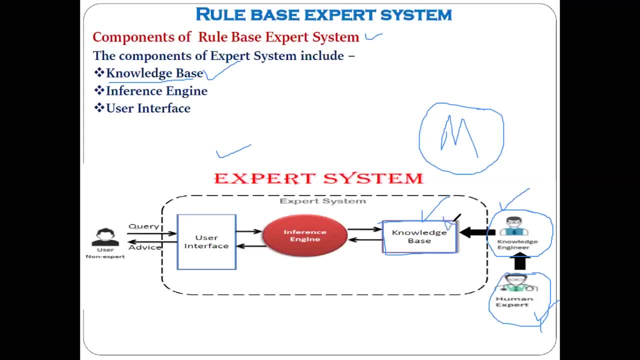 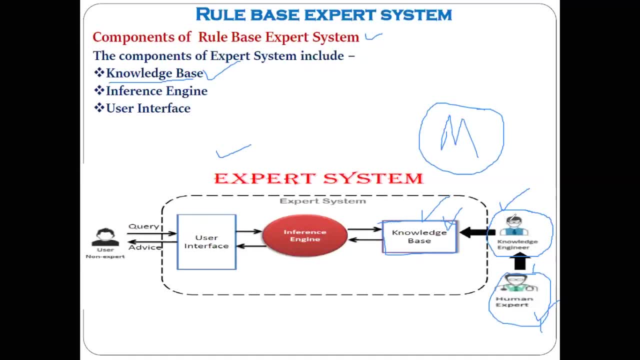 yes or no? who is doing all this? the knowledge engineer, knowledge of engineering. now, assume that we have got our knowledge based. now, now our of you understood what is what does mean by mean by the knowledge base? nja, yes, yes. now next, companies, while the influence indian. 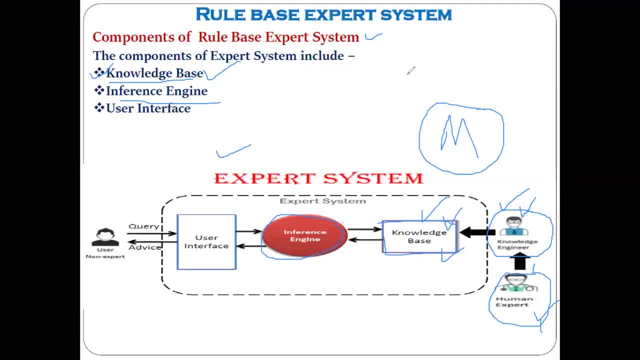 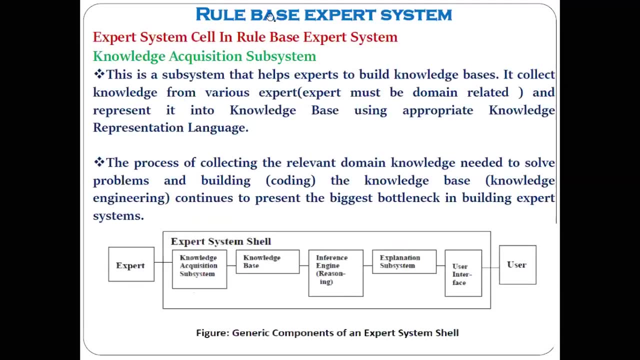 component is what? conference inbro, indian. okay, now let me, let me tell you uh, the, uh, the uh, so um things where I have written here the same thing that we have discussed, So this will be useful for your taking the notes. So knowledge base is nothing but the subsystem that helps. 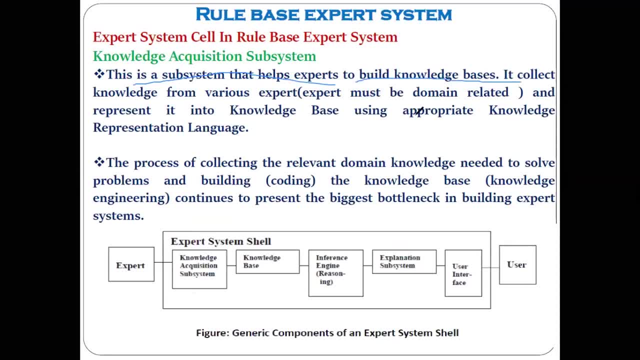 the expert to build the knowledge base, The same thing that we have discussed- Okay, It gathered the knowledge from various expert experts- must be domain related means. what, if you are trying to develop the expert system related with the medical you must, you must. 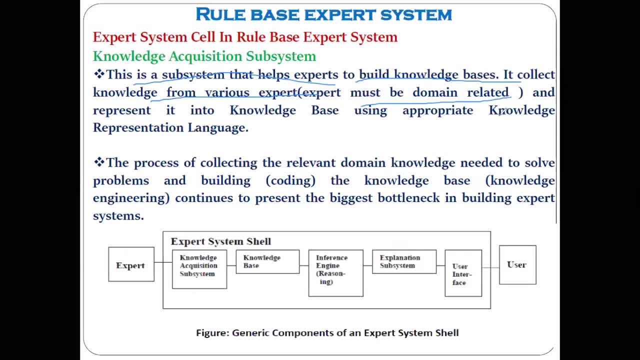 you must gather the knowledge from the expert of the medical only. Correct, That is the meaning of the domain related. Okay, So it collect the knowledge from the various experts. Expert must be from the domain related and represent it in the into the knowledge base. 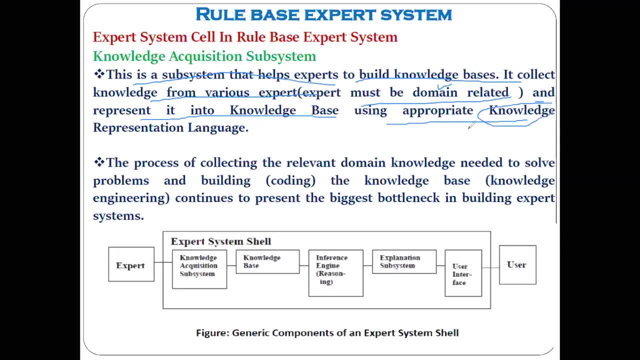 using the appropriate knowledge representation language. So same thing we have discussed. Okay, After gathering the knowledge, it has to be represented using some knowledge representation language, and one of the language that we are going to discuss, we are having to discuss, is the language of the prologue, And that language is called as the prologue for your 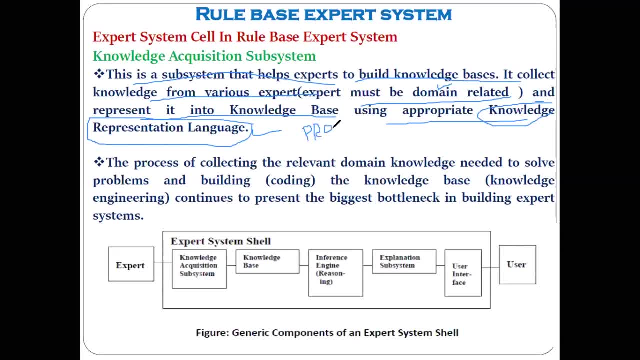 kind information. Okay, So prologue is the one of the language which can use to do the knowledge representation. Okay, Then the process of collecting the relevant domain knowledge needed to solve the problems and building the building, or building the knowledge base in the sense we need to do the some coding for that purpose and continue to present biggest. 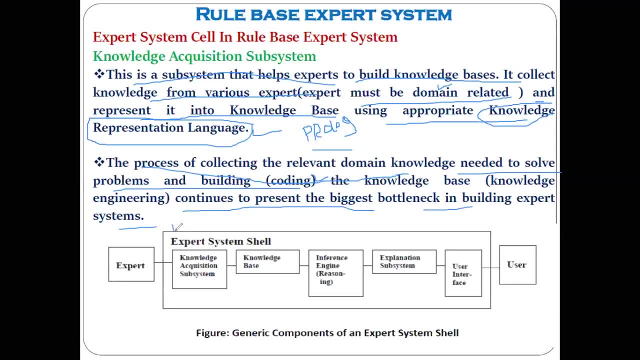 like in the expert system. here also, i have shown one diagram now. this is the more detailed diagram of the expert system. okay, here you can see the same components are there, but some extra components are also there, like knowledge acquisition system is there and- uh, explanation, subsystem are there, yes or no? okay, see, this knowledge acquisition system is related with the 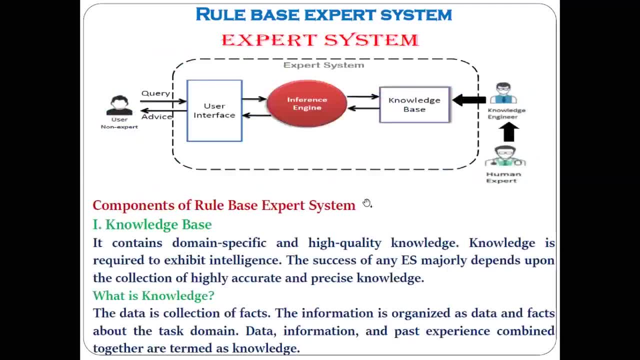 knowledge base only. okay, we'll see that in the next. so here i have mentioned some another point related with the knowledge base. it contain the domain specific high quality knowledge. knowledge is the. now you know what exactly mean by the knowledge that already all of you are knowing. 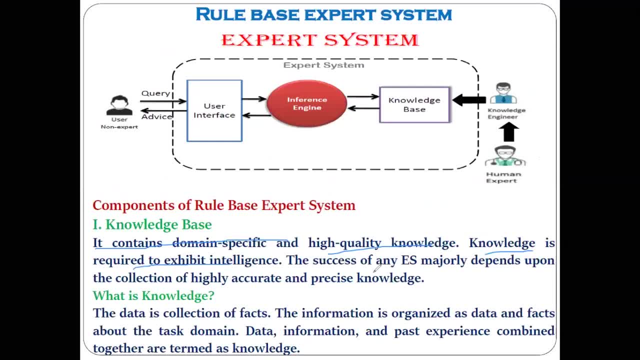 knowledge exhibits there's some kind of intelligence. okay, and the whole success of expert system majorly depends upon collection of highly accurate and the precise knowledge. okay, now if you collect or the, if the knowledge engineer collect the incorrect or the- what we can say- unnecessary knowledge which is not related with the medical field, then your expert system will be also give. 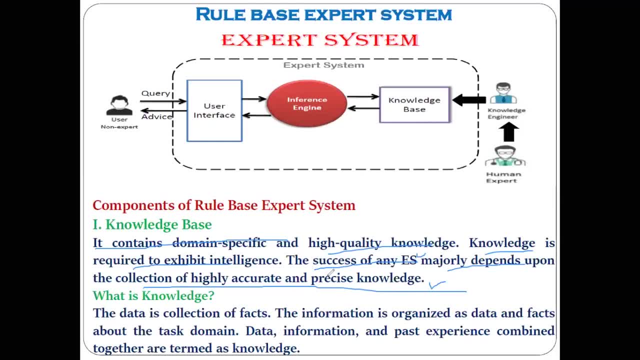 you the result according to that one understood. if the knowledge is incorrect, definitely your expert system will give you the incorrect advice, yes or no, or it will give you the incorrect output, understood. so whole success of expert system depends on the this particular thing: accuracy of the knowledge. okay, now knowledge. what exactly knowledge is that already know? 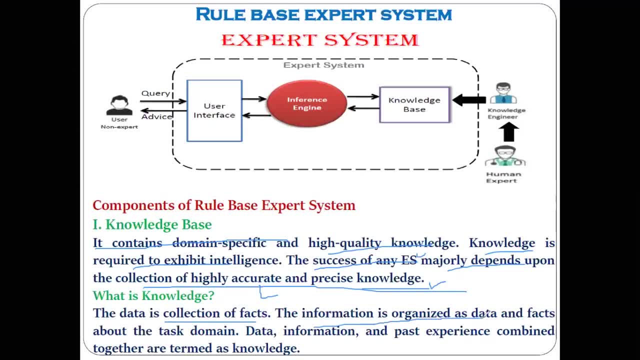 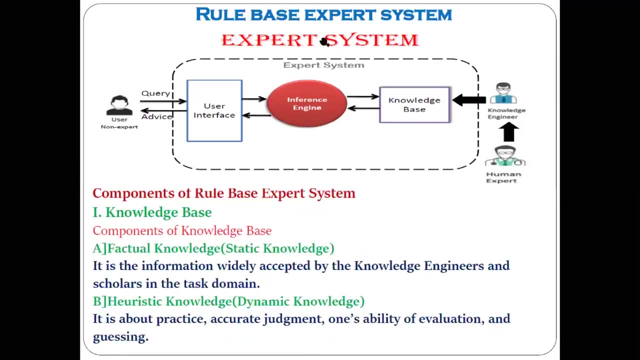 still, I have written. it is a collection of fact. the information is organized as the data and facts about the task domain, and knowledge is nothing but data. information and the past experience combined together is nothing but the codizer knowledge. okay, that all do we have discussed. now there are the two important components of the knowledge base also. okay. 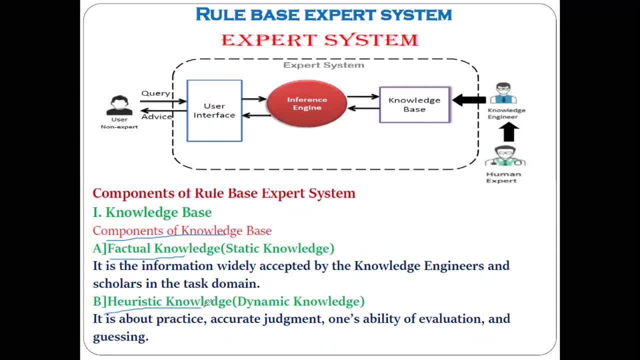 one is the factual knowledge and another is the heuristic knowledge. okay, one is what? factual knowledge, which is also called as the static knowledge, and another heuristic knowledge, which is also called as the dynamic knowledge. now you tell me the any example of static knowledge and you tell me the any example. 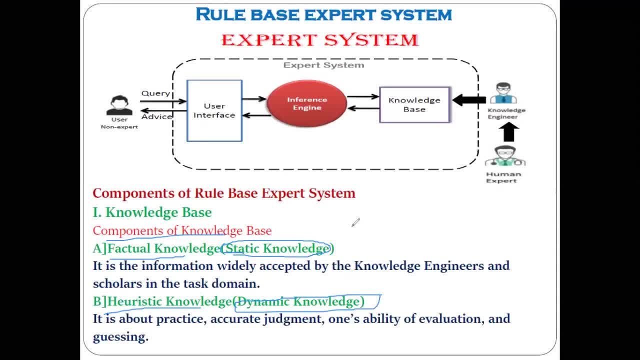 of dynamic knowledge. I want the answer from your site related with this thing. what do you mean by the static knowledge and the dynamic knowledge? heuristic knowledge is good, okay. and the static? What is the meaning of the word? static in the sense, Do not change. Now you tell me from where the sun rises and where does the sunset happen. 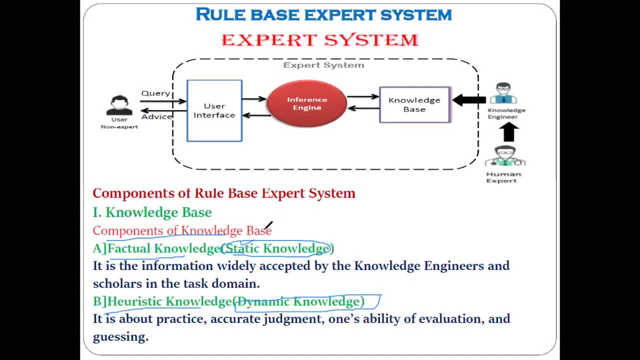 Is it going to be changed? No, No, That is nothing but the factual knowledge or the static knowledge, which is never going to be changed. Change, Change Now. let me give you the example of dynamic knowledge. Now in the classroom, some XYZ student has got the out of 70, has got the 60 marks. 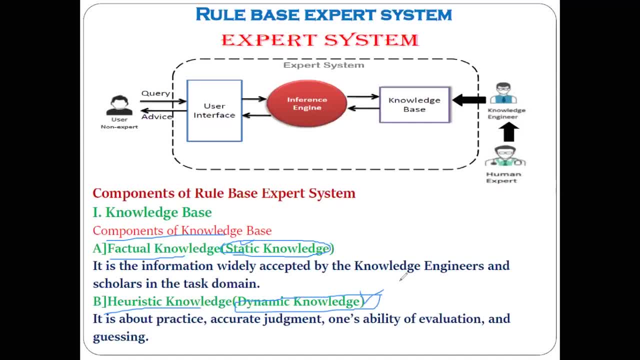 How many 60 marks? But after some time, some days, it is found out that he has done the copy Now, when he has initially got the 60 marks. what is our thinking about that student Now? he is a brilliant, yes or no? 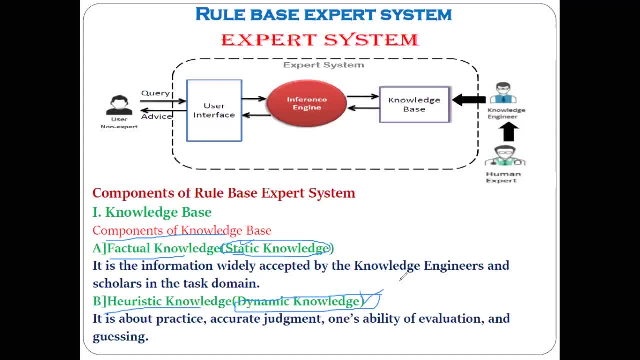 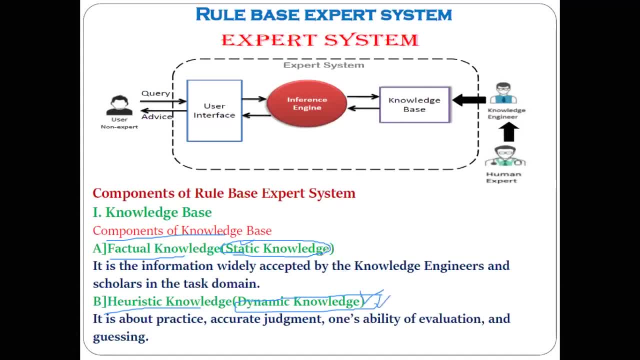 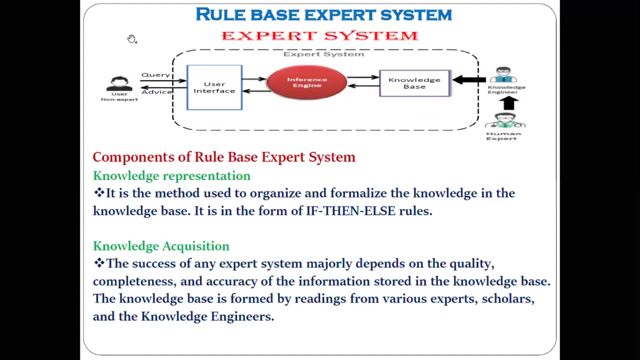 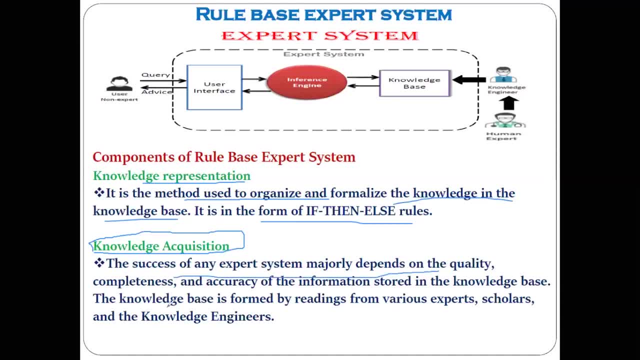 So the success of any expert system majorly depends on the quality of knowledge, completeness of the knowledge, accuracy of the information store in the knowledge base. And you can also get the knowledge base can be formed by reading the various experts or by taking advice from the various experts, scholars, and these all the things being done by whom, the knowledge engineers. 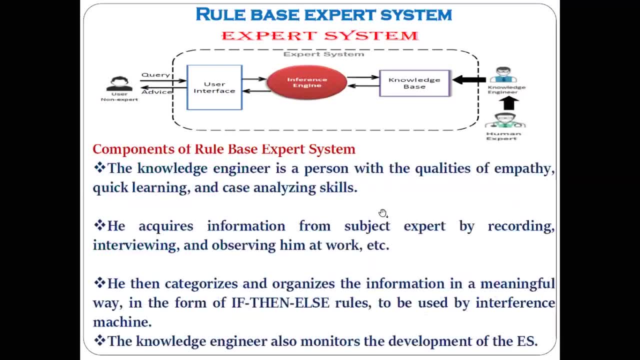 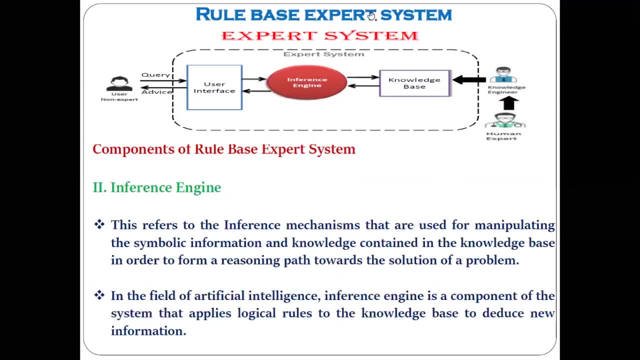 Okay, so this is the first component. I hope all of you got the first component of the knowledge base. Okay, the sorry first component. our expert system, that is what the knowledge base. Okay, this is this much understood First component. Yes, yes, 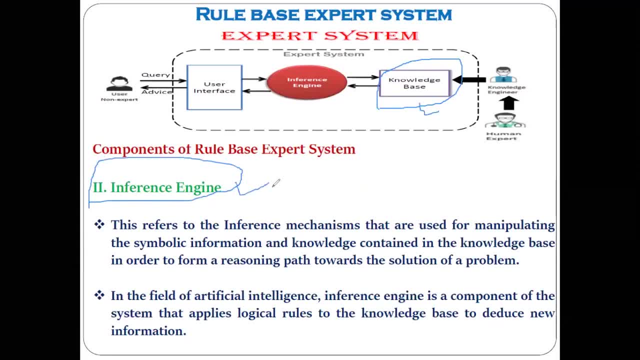 Come to the second component, that is, the inference engine. This is a second, our second component of the expert system. that is what the inference engine Now, what exactly the inference engine does now, when you, When, now, when the we take the same example: natural doctor- Okay, natural doctor, He's a fully experienced, his knowledge basis has form. Okay, he's having the good knowledge, etc. etc. 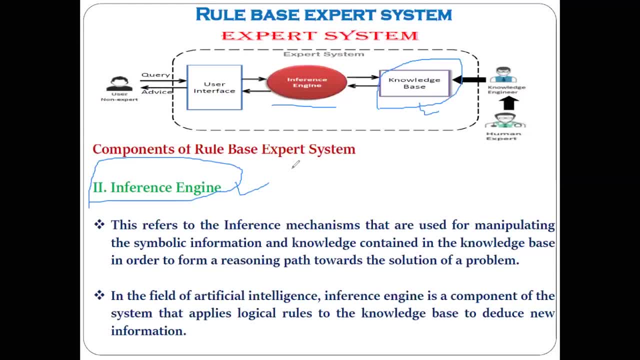 When you go to the doctor and we tell him that, Doctor, I have this kind of symptoms, etc. etc. Now, what he does, he think he think about what you are telling to him- Yes or no. And after thinking, When he is thinking, what he's actually doing. 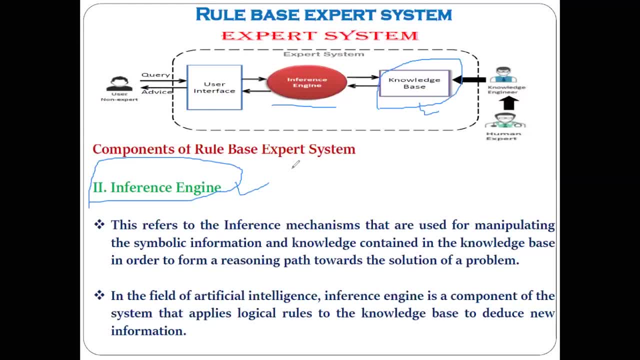 He's trying, he's trying, he's. he's trying to apply his some kind of rules to the knowledge He has, yes or no. What is doing is trying to apply some rules to the knowledge He has got from the previous experience means in the brain- Now I'm talking of the natural doctor. in the brain, The processing is going on, Yes or no. 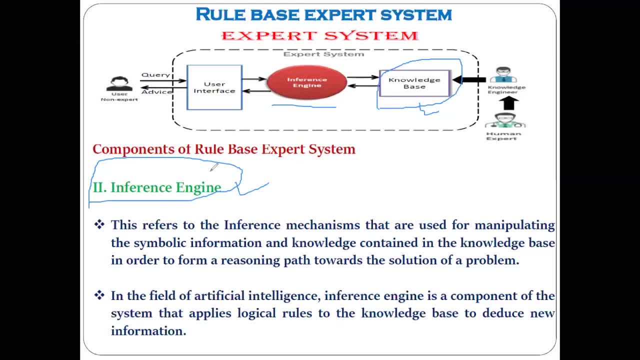 Yes, yes, That is nothing but. and after doing some processing inside the brain, Okay, apply. after applying the rules to his previous experience, he tell you something correct. That is the process, Yes or no? He give you the result that you have this XYZ disease. 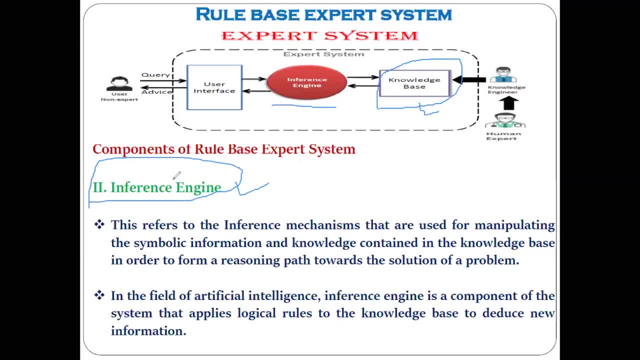 or this kind of disease Means that when he give you the answer, that is nothing but the code as the inference. You got the point. When that physical, natural doctor give you the answer, that is nothing but the code as what the inference. 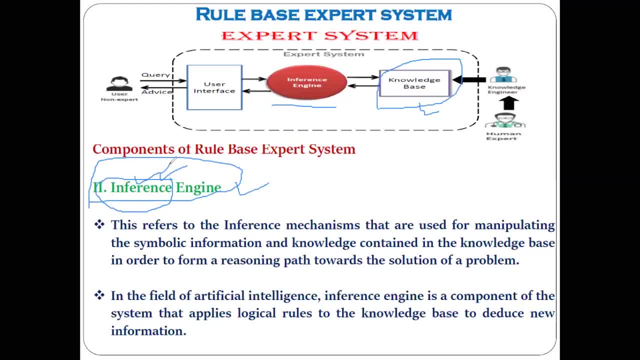 Understood And when we are trying to apply it related with the non-natural expert system. this non-natural expert system has to be built using some programming language code Understood And this is I have written here. this is referred to the inference mechanism. 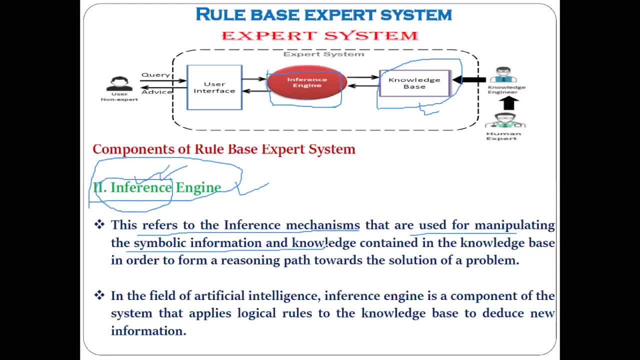 that are used for manipulating some symbolic information and knowledge containing the knowledge base in order to form a reasoning part towards the answer. This is the solution of the problem Understood. So now I hope you have got the what exactly mean by the inference engine. 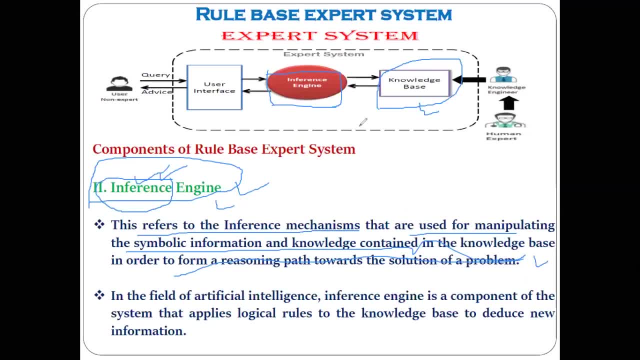 What inference engine does Inference engine apply the rules? where it apply the rules on the knowledge base, Yes or no? Okay, it apply the rules on the knowledge base And from that it try to do some inference. In general, meaning of the inference is nothing, but what? 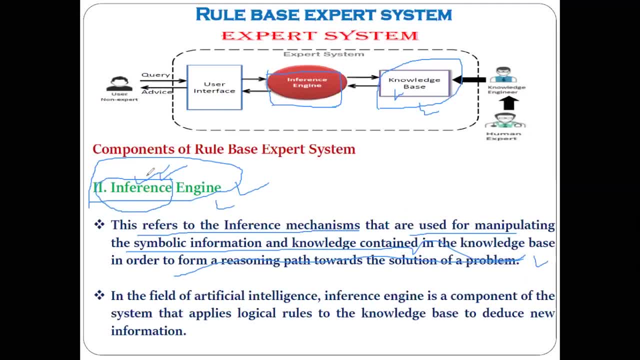 In general, meaning of the inference is nothing but what Doing some prediction, What the point Meaning of the inference is what Doing some kind of prediction, Okay, And then it tells you that you have this kind of disease. In the similar way, 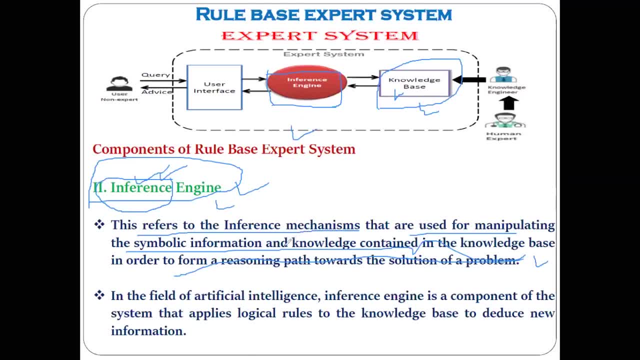 non-natural rule base expert system works. Okay. So in the field of the artificial intelligence, I have written the inference engine description in another way also. Inference engine is the component of the expert system that apply some logical rules. What inference engine? 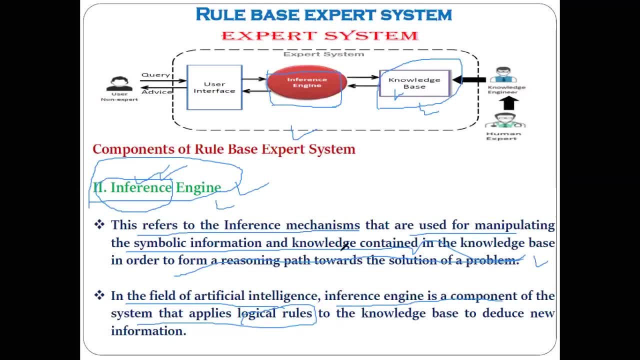 What inference engine? What inference engine does Inference engine apply some logical rules? Where it apply that logical rules On the knowledge base Understood For what purpose it apply the rules to the knowledge base To deduce the new information. 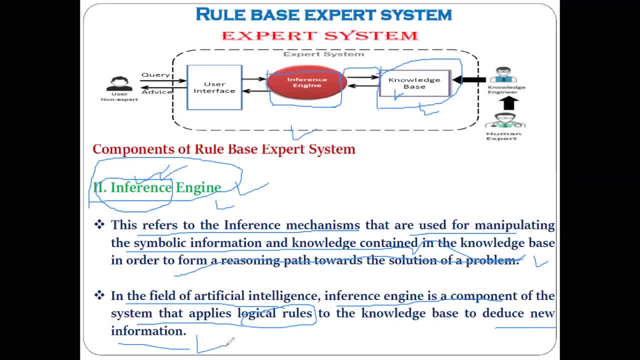 For what purpose? To deduce the new information. What do you mean by the deducing the new information? What is mean by the deducing new information? It means the results. Yes, Did you mean the new information in the sense To get some new information? 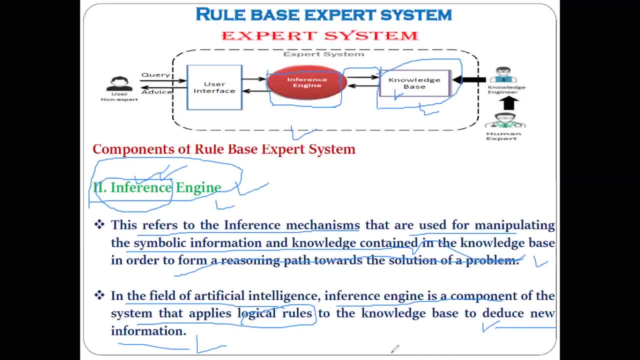 New information Understood Now. when the natural doctor thinking at that time you can apply here, We can relate it to that, that when you are, when that natural doctor is thinking, that in the thing, but it's, it is. 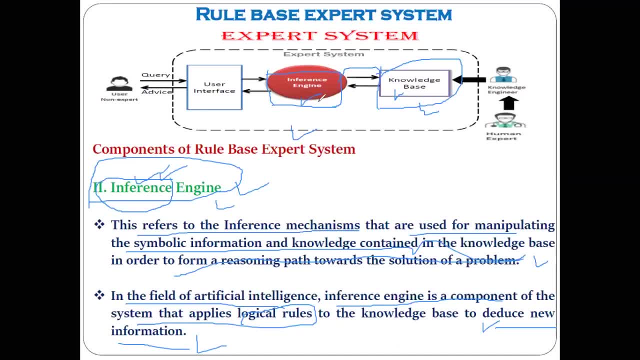 it is, is doing some kind of inferencing, yes or no? got the point: when our natural doctor is thinking about the input that you are giving to that doctor, when he is thinking about something that is nothing but the processing of what inferencing understood, and when we are trying. 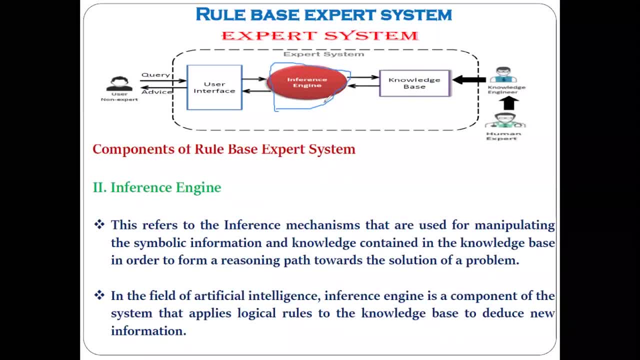 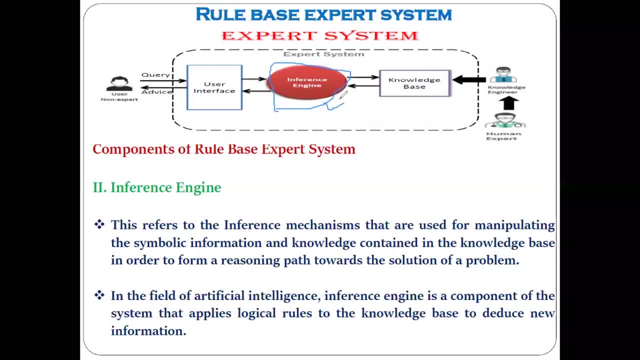 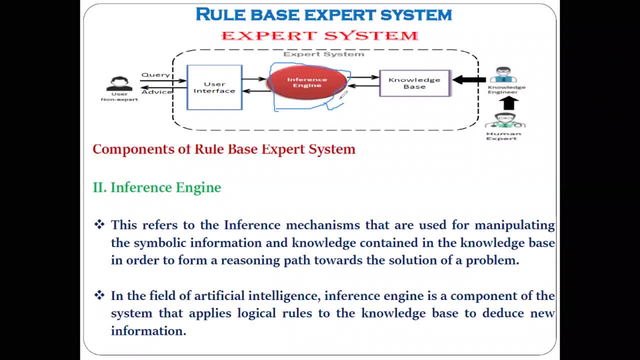 and after thinking, he gives you some output. yes, sir, that is the called as what inferencing, When he is thinking what exactly he is doing? he's, he's, he's trying to apply some, he's trying to fetch his experience. Okay. 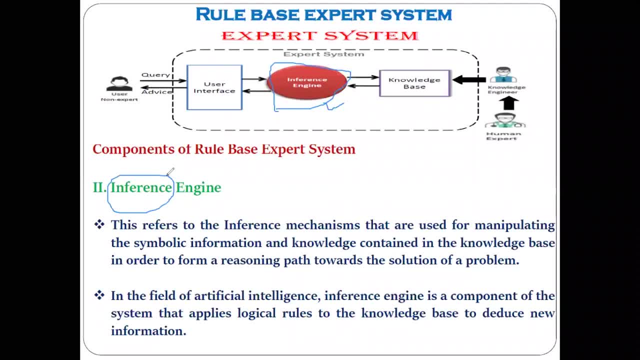 He's tried to apply some rules on his knowledge. What the point? And from that he tell you something. same thing happening here, the inference engine. you can see the arrow from this side to this side You are getting. yes, sir, apply the same example. 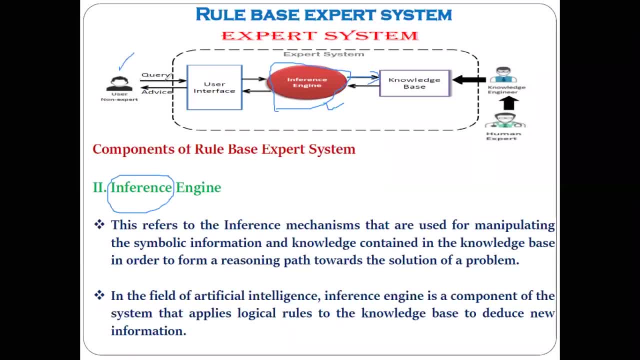 Query goes from the patient or the user as a non-expert query, goes to the. from the user interface It goes to the inference engine- Okay, And then from the inference engine it goes to the knowledge base. knowledge based on the guy, all knowledge, all knowledge gathered. 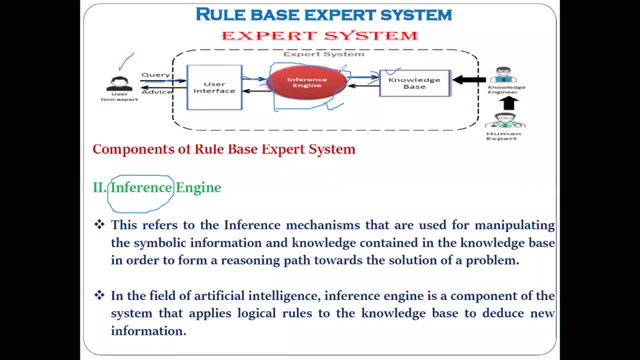 What the inference engine does inference engine compare, compare what query has come from the this user, as we are calling him as a patient. Okay, Yes, And if that query get matching this knowledge base, then this knowledge base gives you the some result. 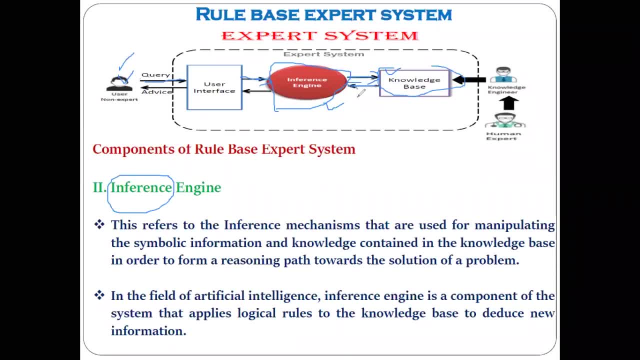 You can see the backward arrow from knowledge base here. Yes, Yes, Yes. Then from the inference engine it goes to the through the some user interface. again it goes to the as an advice to the user, as a non-expert. yes or no, same thing happens. 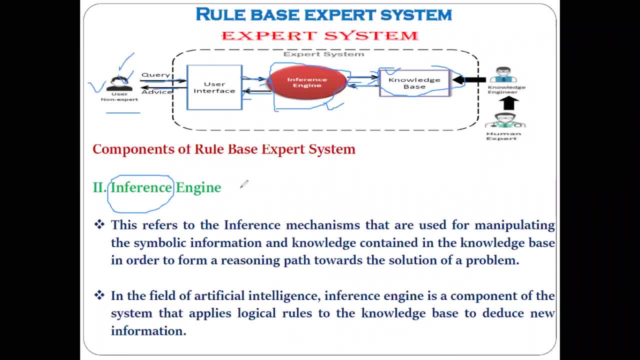 when you go to the doctor. Okay, In the hospital, Correct? Yes, That is the thing I have written here. It refers to the inference report, to the mechanism that are used for manipulating the information. manipulating in the sense processing the information. 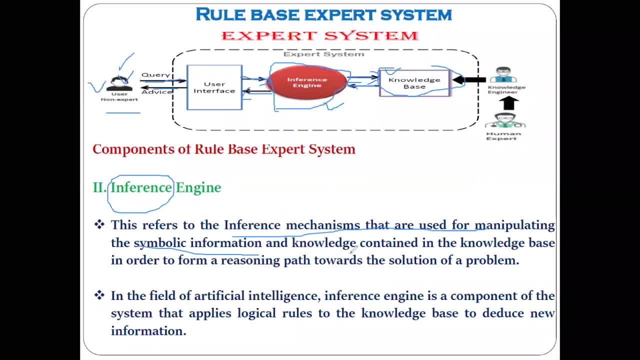 Got the point Okay, Manipulating the information and the knowledge content in the knowledge base at the doctor's knowledge base Brain. Yes, Yes, Yes, Yes, Yes, Yes, Yes. This is a knowledge base guy, a non non-natural expert systems up on programming through using 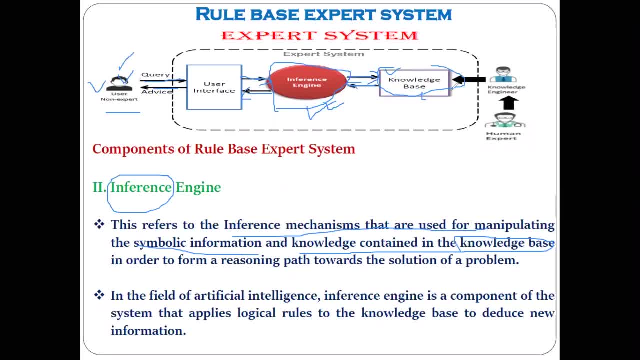 database. We are doing uh here here using some database, We are creating that knowledge base, correct? Yes, sir, Yes, So this is nothing but all the things related with the knowledge base, the second component of the what you can say, the expert. 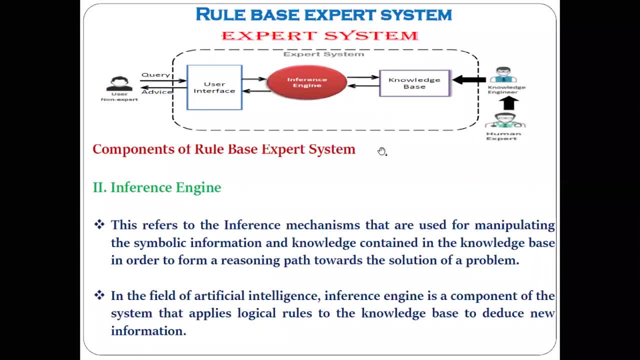 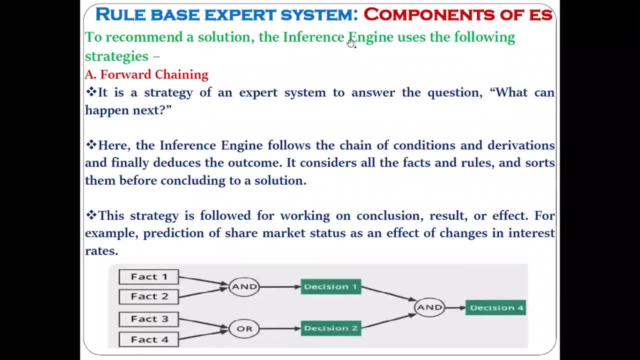 Yes, Merci Now, and let's see the next point. Now, inference engine can give you the okay, can give you the result with the help of the two important technique: okay, or the expert system, or the sorry. inference engine can. 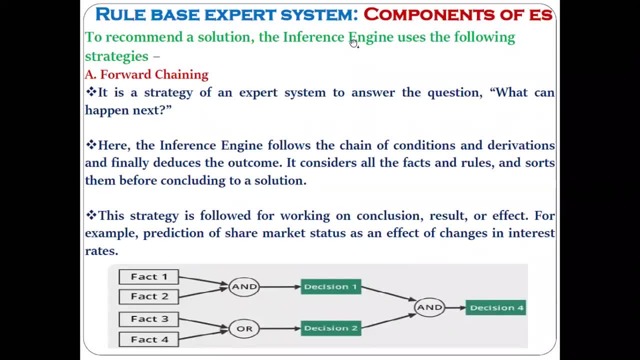 give you the solution with the help of the two important technique. on this technique, separate question being asked number of times- okay, one is that the forward chaining. okay, one is what forward chaining? and another is the backward chaining. now you can see this. 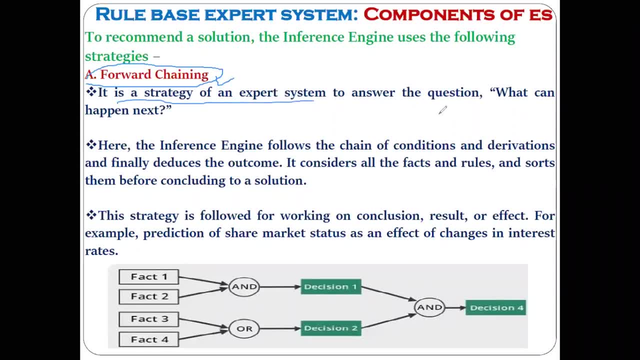 but forward chaining is the strategy utilized by the expert system to answer the question. now, what does it actually mean by the forward chaining? now, forward chaining simply gives you the answer related to the question, like: what can happen next? What? forward chaining is simply what can give the answer related to the things: what? 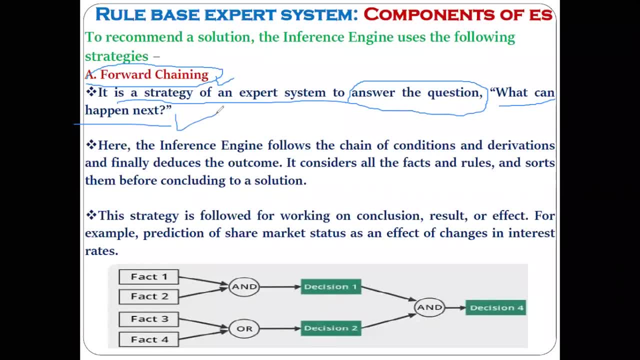 can happen next? let me give you the example. now you are at the home and you see the environment is fully cloudy, humid environment. is there? what does it mean? rain come, rain might come. rain has not started yet, but rain might come. yes or no means yes or no, rain might come. 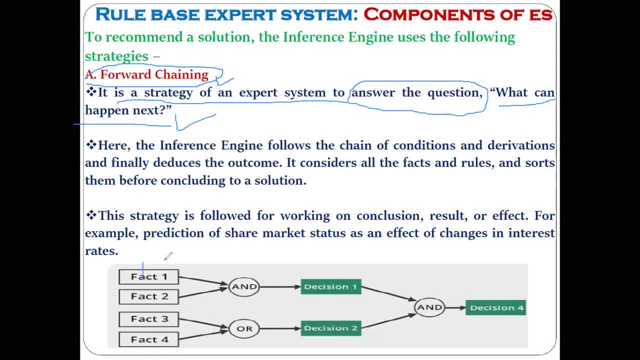 you know some fact. see the figure. you know some facts, facts 1,, 2,, 3,, 4, etc. correct what fact? you know that environment is fully cloudy, humid. that are the facts. correct now from that facts can you take some decision? what decision you can take? suppose you want. 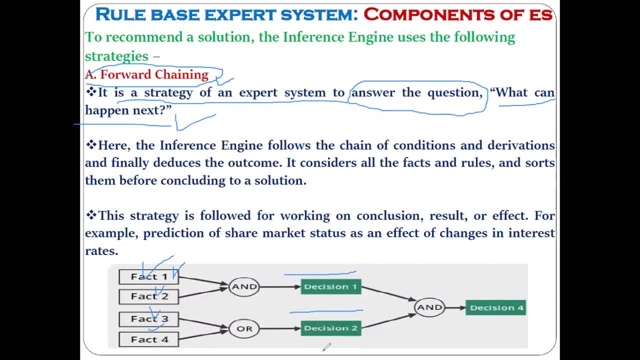 to go outside. what decision you will take On the right, On the left, On the right, On the left, On the left? We should not go outside, But suppose you want to go outside, Then we can use umbrella. umbrella, that is the decision. umbrella, yes, yes and from. 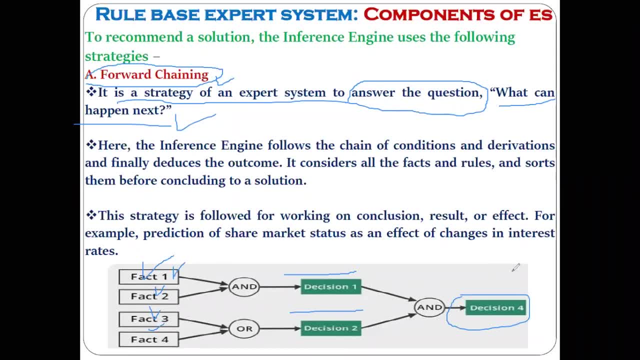 that you reach to the some goal, that you, you take the umbrella and you go outside. yes, understood, and that is the reason it is called this kind of this kind of what you can say solution is called as what: The forward chaining. 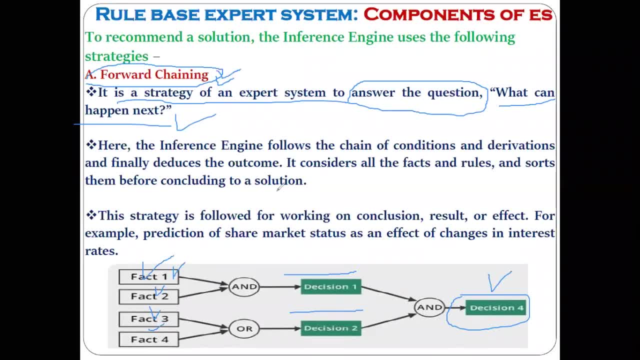 Okay, Okay, understood. what does it mean of the forward chaining? yes, sir, it can give the answer to the what can happen? next question now, how it can give the answer based on the known facts. understood, yes, sir, okay, so here the inference engine follow the chain of condition. 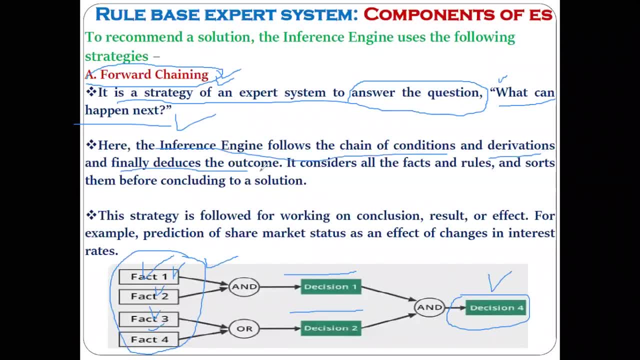 and derivation and finally he can predict the outcome. okay, and it consider all the facts and the rules and sort them to calculate the solution understood. so this strategy followed for working on the conclusion, result effect, etc. etc for doing the different kind of prediction. now this is the 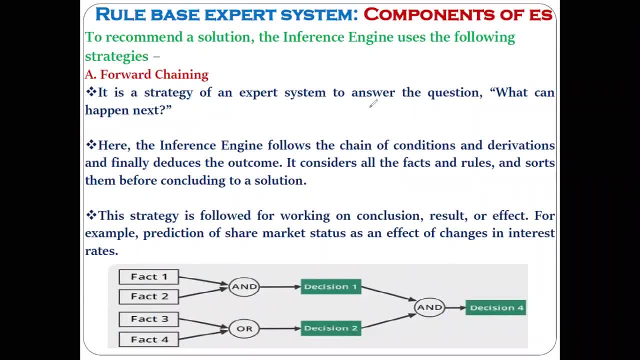 one way of providing the solution. okay, inference engine can use the forward chaining. okay, that is the one way okay to perform the processing as we have discussed. inference engine does the processing okay, by comparing the facts with the knowledge base. okay, so forward chaining is the one way. another way is the backward chaining. now it is opposite to. 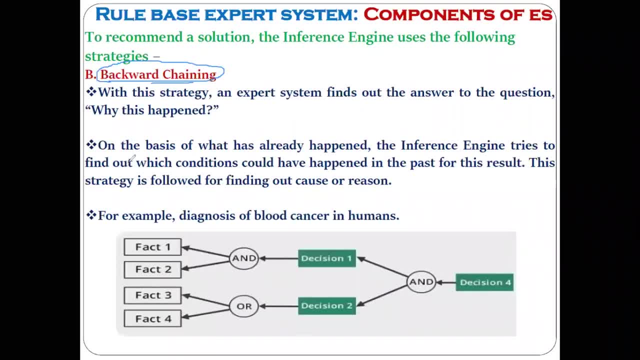 the forward chaining. another way of providing the solution is what the backward chaining? so it can give you the answer why this happened, what it can give the answer to the question like why this has now, as I said, is opposite to the forward chaining. in the forward chaining, what is happening? we start. 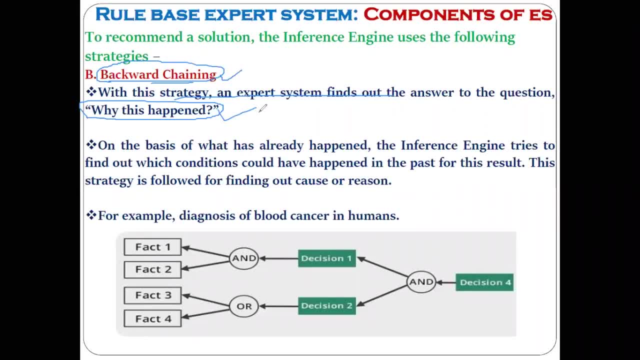 from the some fact and we reach to the goal. we reach to the goal in the sense you take some decision, understood, yes, yes, yes, sir, now tell me about the backward chaining. forward chaining was what fact to the decision? correct opposite to the forward chaining is what backward chaining? so it can be? what decision to the fact? 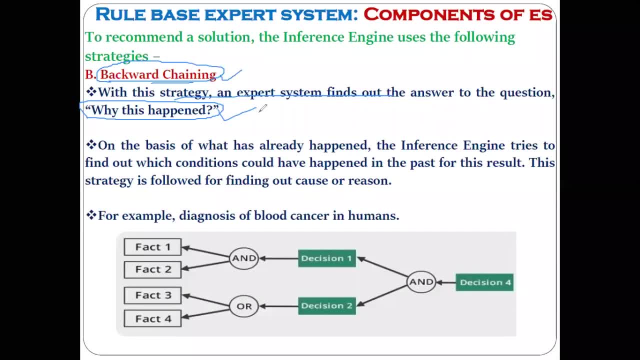 yes or no? yes, yes means if you consider the forward chaining as an initial state to the goal state, then can we consider the backward chaining as a goal state to the initial state or can we consider this is a from decision to the fact- reverse to the backward chaining, that is. 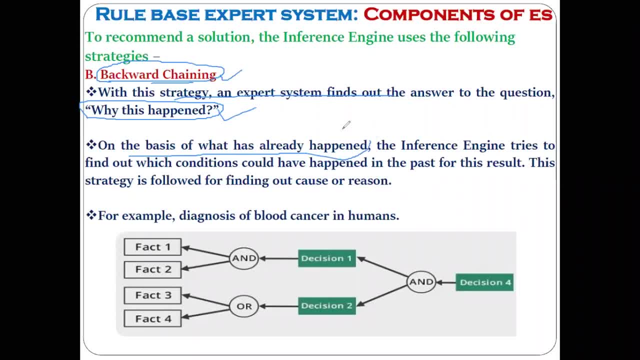 nothing but the backward chaining on the business. what has already happened? what? on the basis of what has already happened, the inference engine tried to find out which conditions could have happened, done in the past, for these result in the forward chaining, what with the help of some facts. 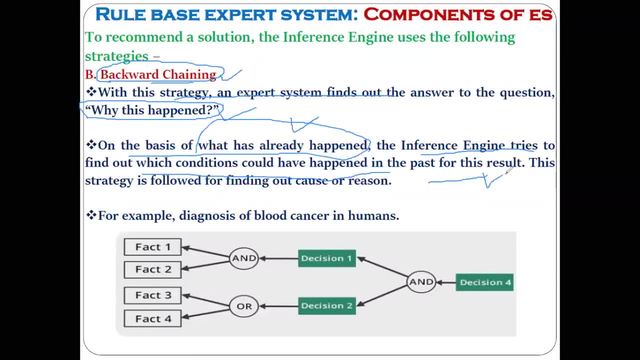 we are trying to reach to the result. yes, in the backward chaining, reverse to that from result, we are trying to reach to the fact or to the condition, correct. let me give you the example now. corona disease have had come first, yes or no? yes, all of you can see the 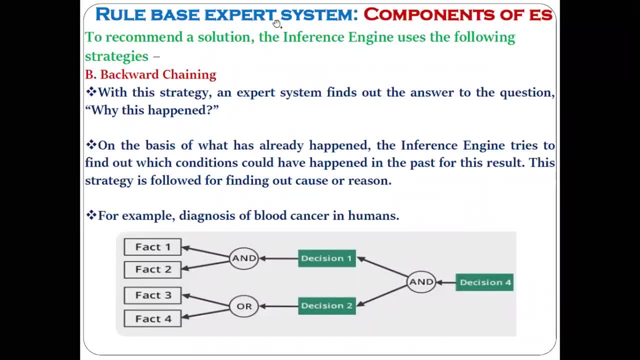 screen. I can't see. yes, now all of you can see the screen. yes, yes, now corona disease has come first, yes or no? yes, sir, after corona disease gets spread out everywhere, we come to know what are the symptoms of the corona disease, yes or no? yes, is it the backward chaining? yes, sir, exactly it is the backward. 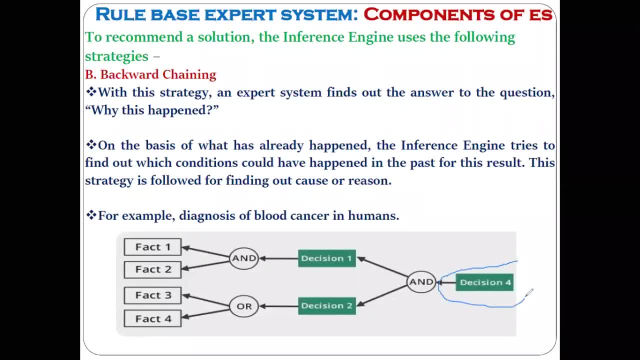 chaining. first we come to know that corona disease has been there, and after that we come to know that these are the various facts or the symptoms because of which corona is happening. got the point? yes, sir, yes, so that is, but the backward chaining. this is a very important point: forward chaining and the backward chaining. 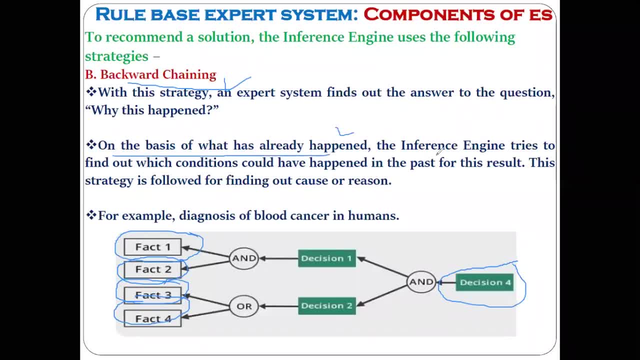 so, on the basis of what already has happened, the inference engine tried to find out which condition could have happened in the past for this reason. and the back forward chaining is what? completely opposite to these things? on the basis of what? on the basis of facts, forward chaining. 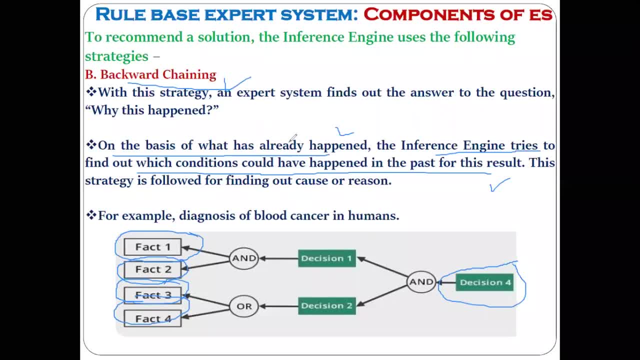 try to reach to the conclusion, okay, but the backward chaining from the conclusion it tried to reach to the fact understood, yes. so on the basis of these two technique, the inference engine, try to compare the things with the knowledge base, and if you try, then it try to give the solution to. 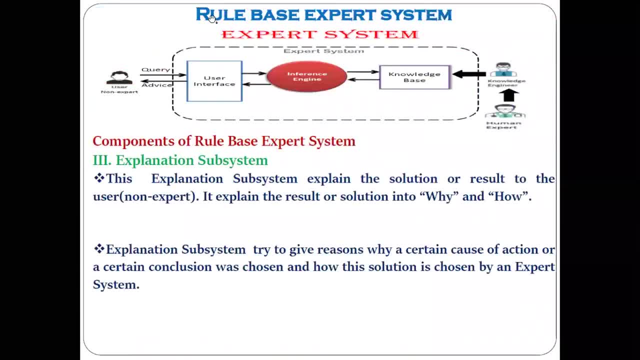 the user as a non-exploit- okay. now, another component is their explanation subsystem. okay, in that diagram, another diagram i have shown you here, in this diagram i have not shown in detail explanation subsystem- now it explains the solution to the this user. okay, in order to, in order to explain the solution to the user, there is a utilization of the. 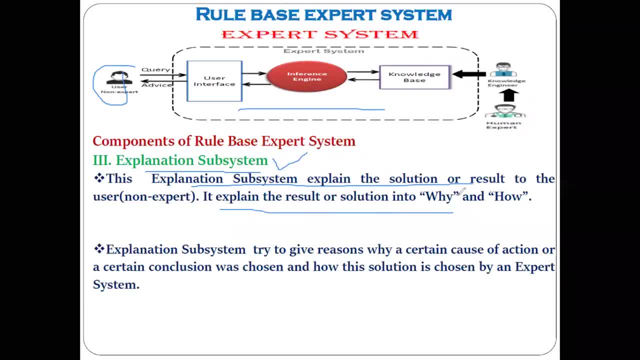 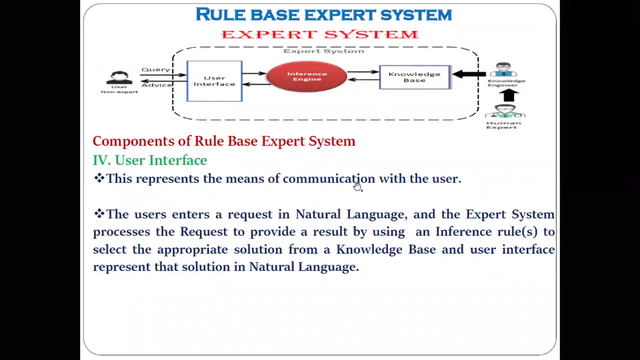 explanation subsystem. now it explain what, why this has happened. okay, and how is it can happen. this kind of, this kind of answer is given by the explanation subsystem. after after now, let me tell, let me take you to that detailed diagram and i'll show it to you. okay, here is the explanation subsystem. 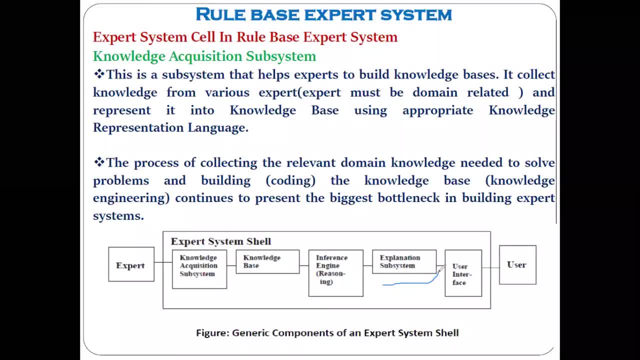 right here. here you can see the explanation subsystem. okay, now, this diagram is a opposed to that, our main diagram. but you can see here after something, here after something comes from the inference engine. okay, here, expert from the expert, knowledge acquisition happen. then from that knowledge base get created. 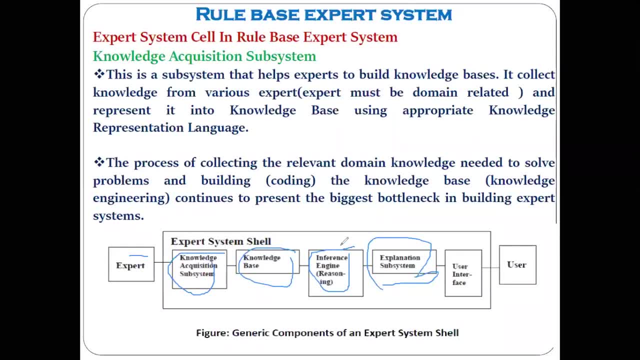 when the knowledge get created, then inference engine get created and then the explanation subsystem. now, when the user asks some query through the user interface, okay, then that that query, through this explanation subsystem- now here explanation subsystem will explain, or will try to try to explain, this query to the inference engine. what the point, then inference? 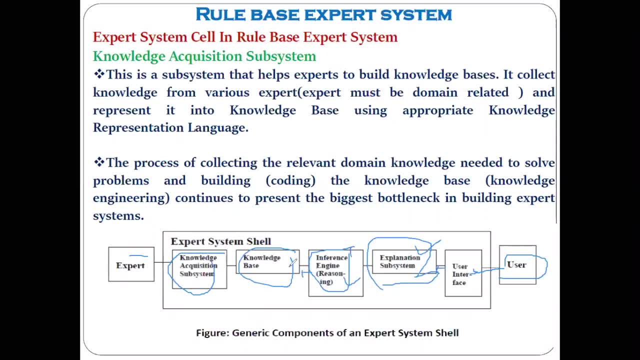 engine send this query to whom knowledge base understood. then after comparing, comparing that query with the knowledge base again, knowledge base will send answer to the inference engine. then inference engine send that back to the explanation subsystem and then explanation subsystem subsystem through the user interface own tell it to the user what the point. so explanation system work between the inference engine and the 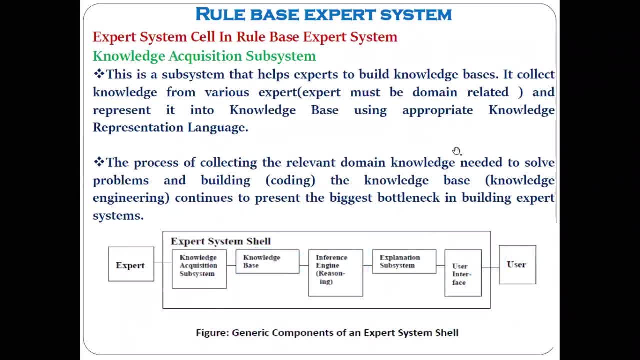 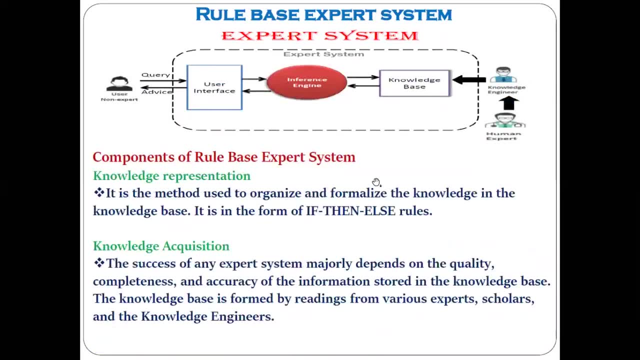 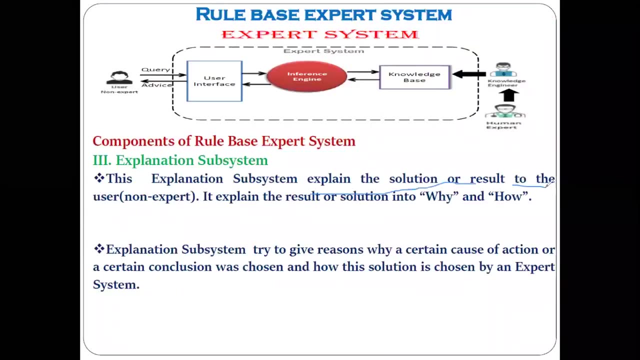 user interface. it can. it can tell to the user or it can tell to the inference engine related with the solution. okay, here I have mentioned okay, here you can see the explain system, explain the solution or result to the user or to the non expert in detail diagram. you can see that okay. 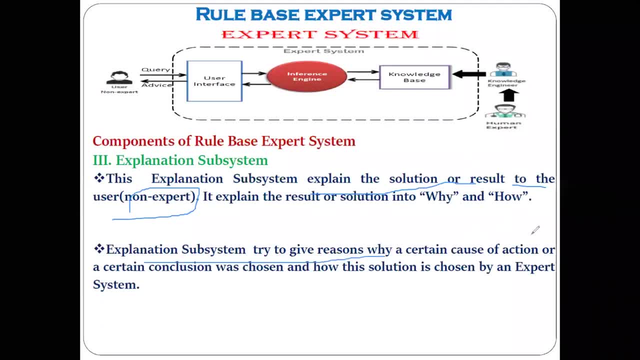 so explain subsystem, try to give the reason why certain, why, what? what is the reason of certain cause of action or what is the reason for certain conclusion, etc. etc. understood, just like when doctor tells you that you have this disease, then you ask your doctor why, why this has happened. yes, 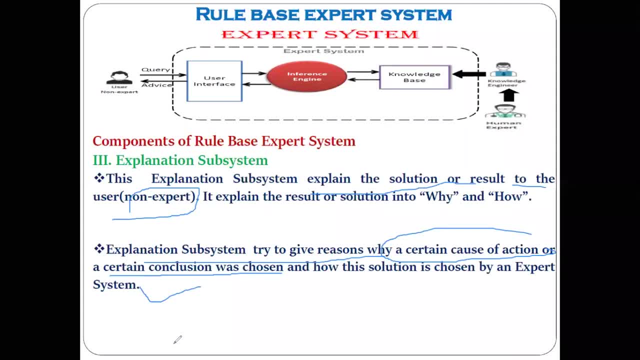 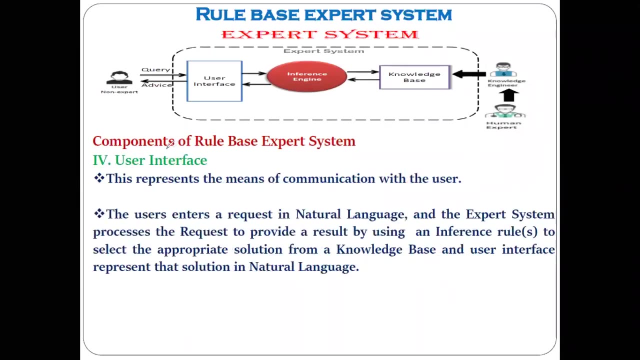 or no. then doctor tells you the reason behind that. what the point? that is nothing but what explanation? subsystem understood, yes, sir. okay, yes, sir. let's see the last component here, the user interface, which already we have discussed. it represents the mean of communication with the user. user, just like i told you you, you go. 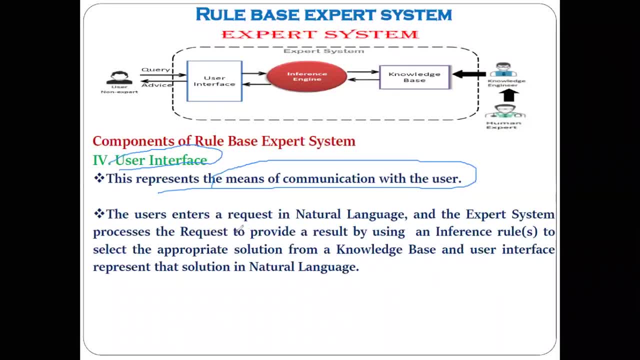 to the doctor and you tell him that what is what? what happening to you? okay, the here i've written. the user enters the request in the natural language and expert process: the request to provide a result by using the inference role to select the appropriate solution from the non-expert. 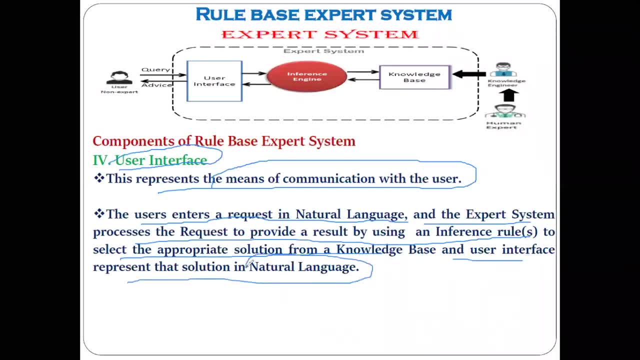 knowledge base and user interface represent that solution. in the knowledge base you ask query to the doctor in the natural language and doctor also tells you the answer of that query in the natural language. the medium of communication between the doctor and the patient is nothing but the called as the user interface. okay, and here, here also, if the non-natural 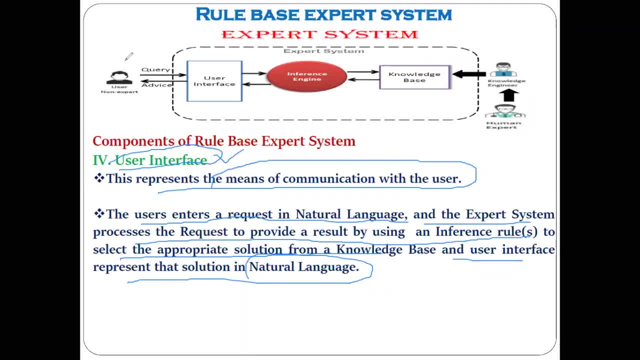 expert system as a software has been developed. consider: the software has been developed, understood. now we understand. in short, whatever we have discussed now. now we have gathered the knowledge base. the inference engine has been created, understood, user interface component has also been created. okay, yes, you are getting what i'm saying. yes, sir, what i said: knowledge base. 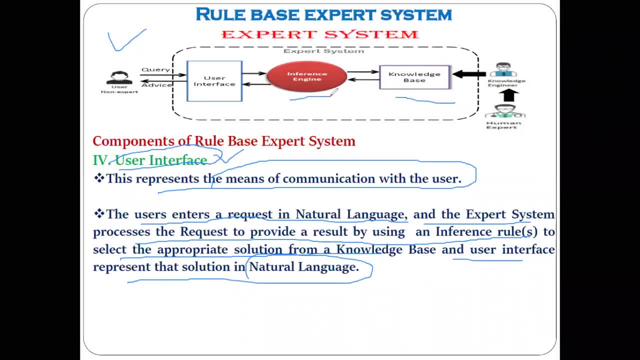 is created. we have discussed what is knowledge base inference engine also created. we have discussed what is inference engine and user interface also created. okay, then, means what? your whole our software system as a expert system is created. got the point? yes, sir. okay, then you want to ask some query to the your now you want to ask some query to that software. you does the. 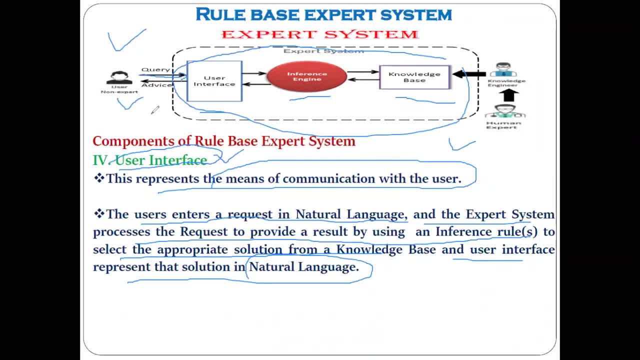 query for the software and you want to know the query for the software or you want to from here. here I have shown the user non expert understood how you does the query. you use the keyboard, mouse, etc. etc. and you write, you type something in the natural language, correct? 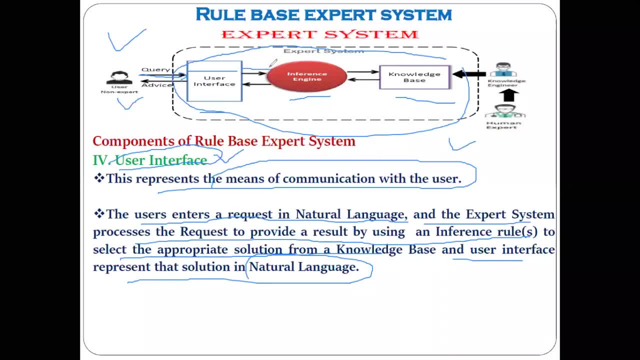 then that request goes to where inference engine. now, what inference engine will do? tell me what will inference engine will do. inference engine will synchronize what is the query and in search in the knowledge base. yes, that inference engine understand what is the query and then it try to compare it with the knowledge base- knowledge base. then what will happen? 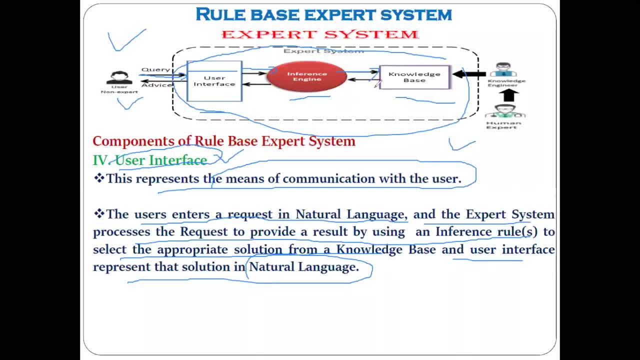 and then it will get the information or the. so if that query get, get matched with that knowledge, what is being here? then what will happen? it's saying the result back to home, back to the inference engine, understood inference engine. check here whether that answer provided from the knowledge. 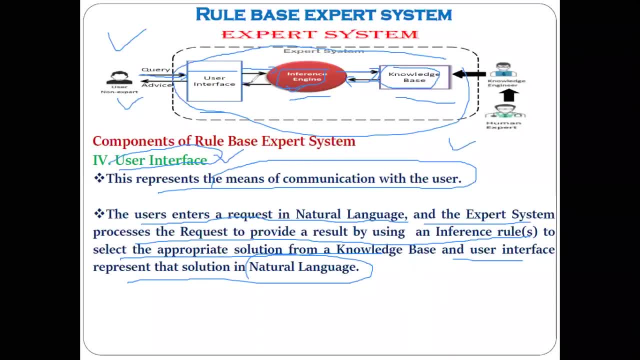 base is according to the query and then inference engine through some user interface It send back to the user as a voice: yes, and this is what rule base expert and the component of the rule base expert system got the point. yes, any query. this I want you to ask. 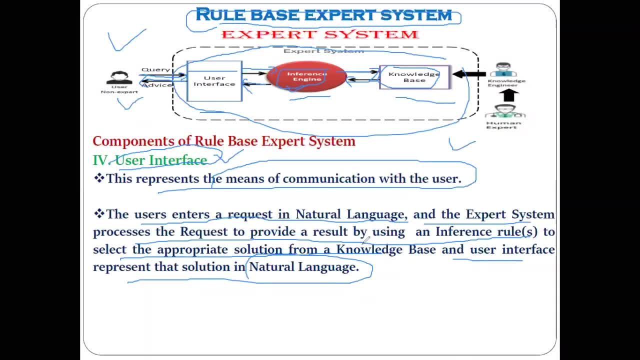 Because now you are not in front of me so that I can read your face. I can and I can conclude that you are understood or not. so here, until I- not, I will not get the response from your side, I cannot take any decision whether you are understood or not, and so that's. 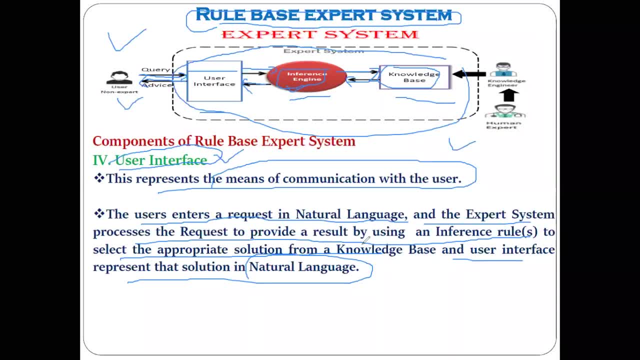 why I need the quick response from your side, whether understood or not understood. you are getting what I'm saying, yes, already. we are getting the problem, while these online teaching and not giving the Quick response. you are adding in that problem, Yes or no. so try to give the quick response, whether understood or not understood, so that 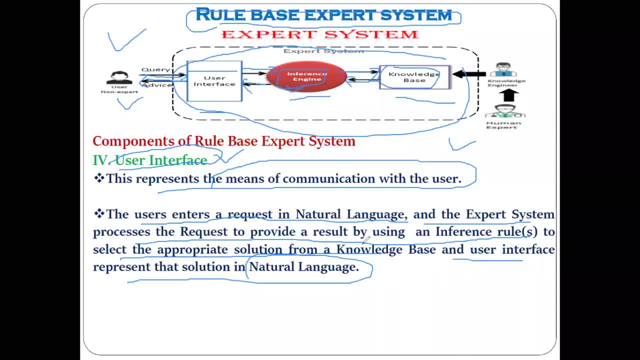 I can clarify it, If you are. if you are, I am asking and you are not speaking anything. it is simply you are consuming the time, Yes or no, Shubham? so try to give the response. whether understood or not understood will clarify it here only. 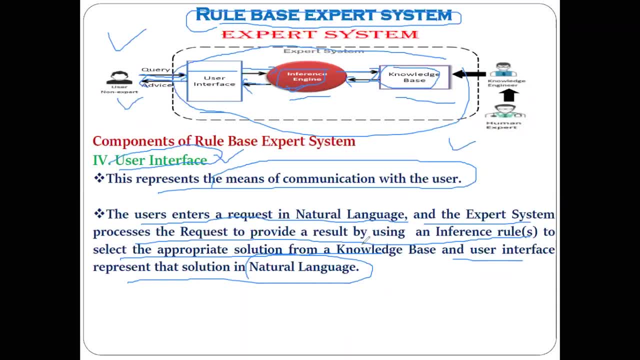 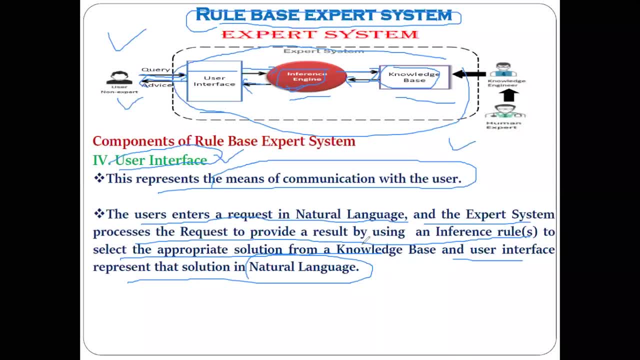 base? Yes, Then what will happen Then? you will not get the result. rule based expert system are having some limitation, correct? Okay, Yes, It. we cannot never get the hundred percent result as compared with the natural doctor. Yes or no? 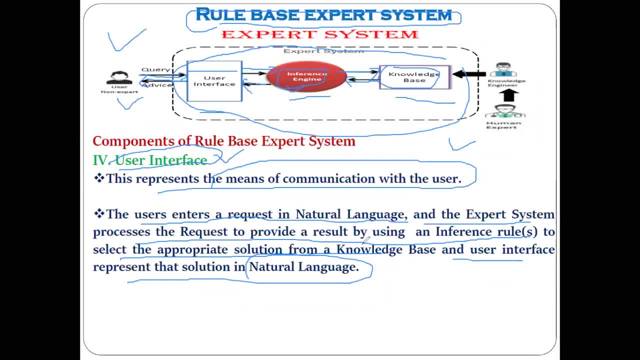 Yes, sir, It is a fact, because this rule-based expert system based on the AI, these are also having some limitations- You will get the answer of that question only- which are being related with the information. is including the knowledge base, yes or no? 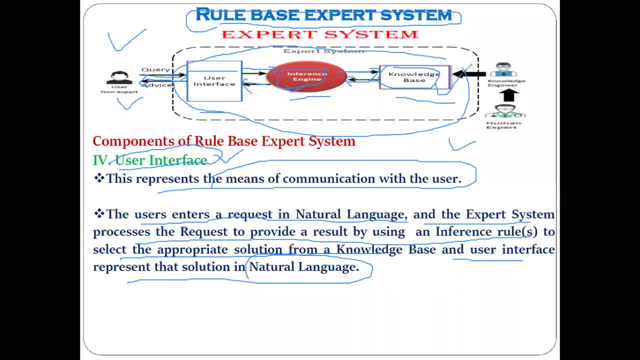 It is replicating the same. If I ask you the question, if you know about that things, then only you can answer me. If you don't know, will you answer me No? No, It is same Right? Yes, sir. 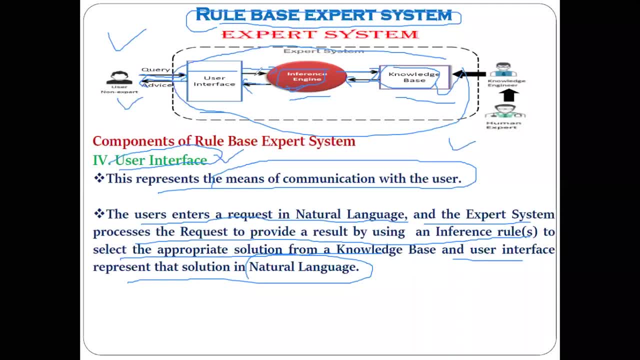 Got it, sir? Yeah, The way you develop it accordingly, it will work. Hmm, It is a fact, Sir. Hmm, Sir Yes. 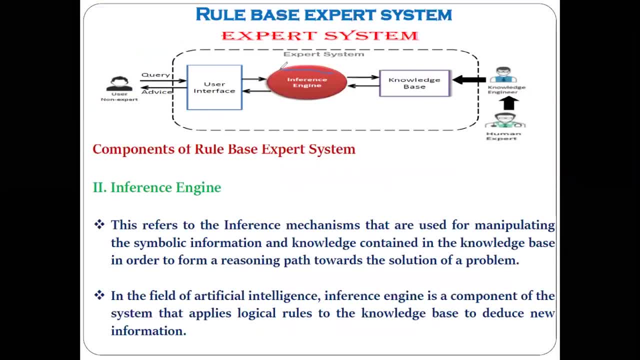 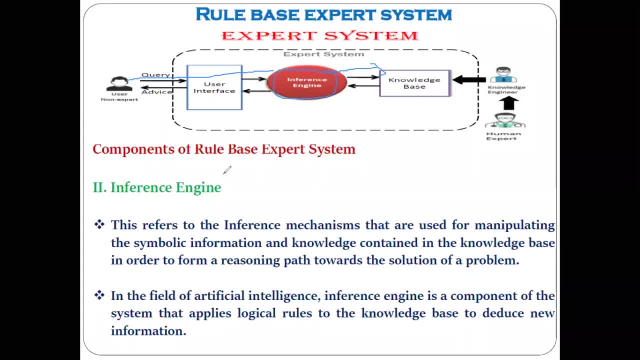 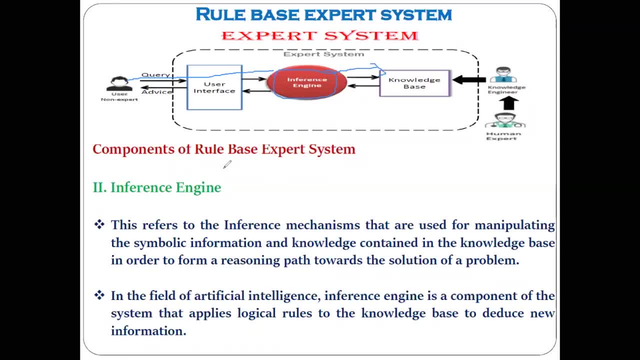 that thing already happened with you. After this thing happened with you, you are trying to find out what are the reason for that. Just like, let me tell you the another example: You are driving the bike and you got instantly. you got accident. Then, after happening of 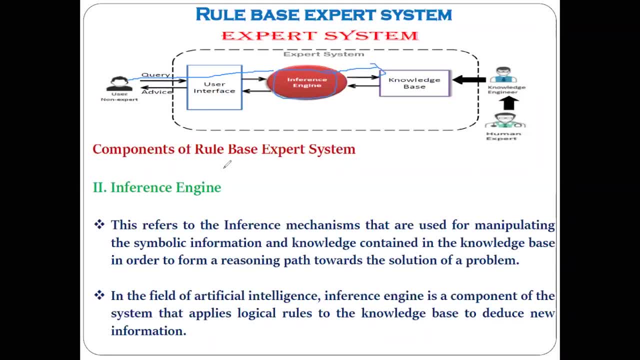 accident. you try to find out how it has happened, why it has happened, what was the wrong. And I have told you the example of that: Corona also, After Corona disease spreading, it has already put his fingerprints in the world. After that we find it out because of what. 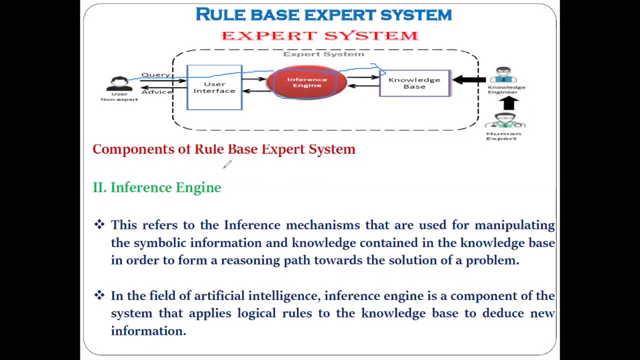 it is happening and what are its symptoms? That is the backward chain. Crime investigation is also backward chain. Yeah, So inference engine works in that way. Understood According to the what kind of query it is getting. Yes, sir. 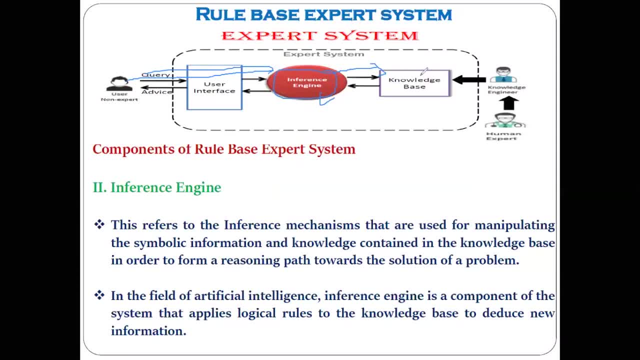 Understood. Yes, Yes, sir. So in the next point also we are having the point related with the forward chaining and backward chaining, that is related to the forward stack planning and the backward stack planning. Okay, That time also we'll try to clarify it more. but here in short, 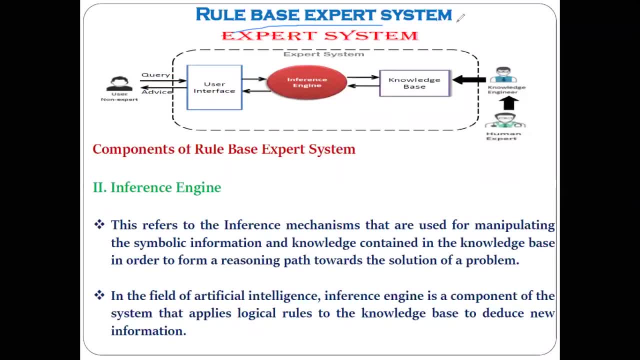 I explained you related with the rule base. This is a very important point from the second minute. So the number of times question being asked on this point: Okay, Instead of asking directly the component wise question also being asked number of times, like knowledge base inference.